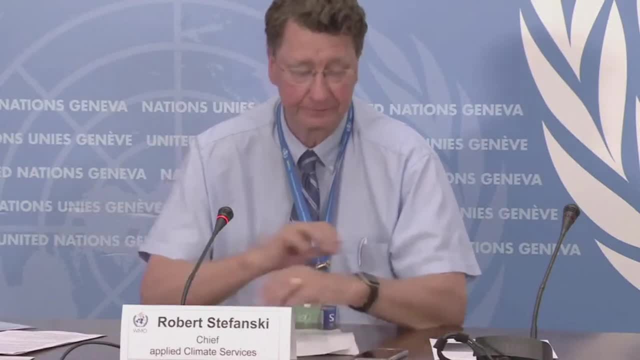 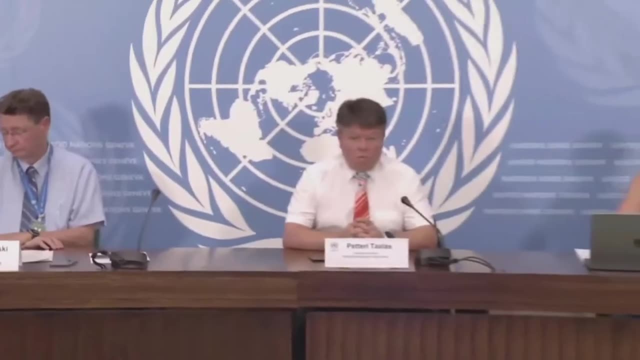 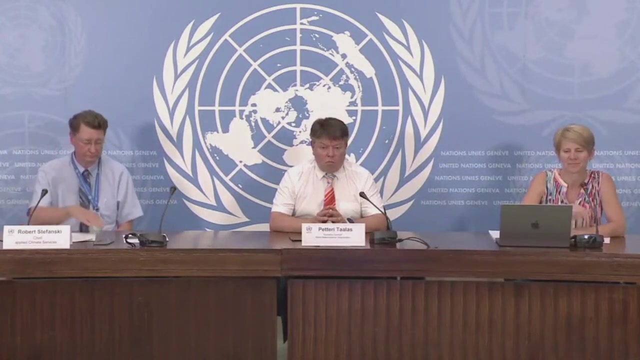 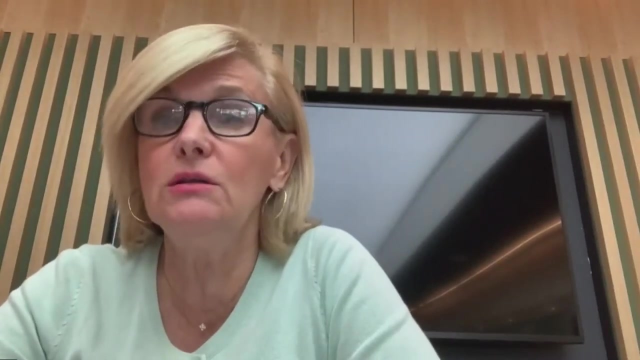 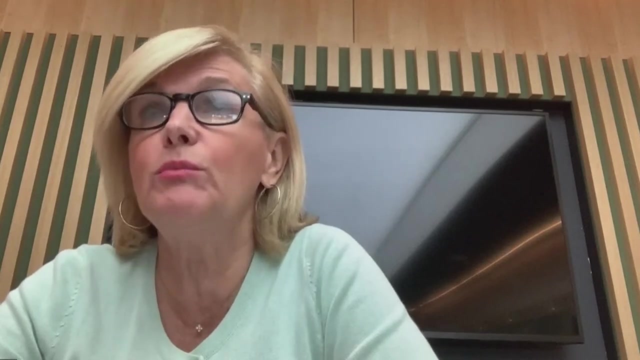 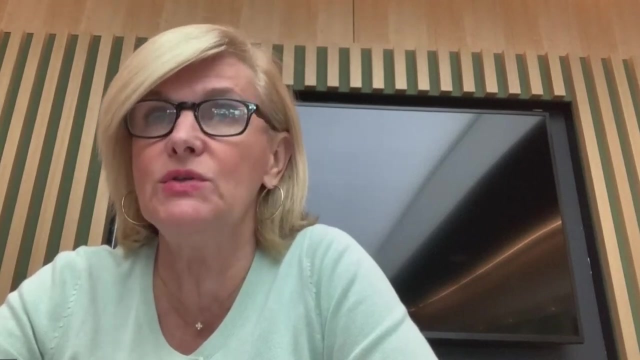 the next three or four weeks. Thank you, Thank you very much, And now I give the floor to Maria Nera, Director of Pharma. Thank you very much And a pleasure to join you today. I am in London at the moment where the mayor of London, together with the World Health Organization, is hosting a solution summit on air pollution and climate change. So, as you can imagine, being in London today at 41 degrees is so exceptional, You see that. 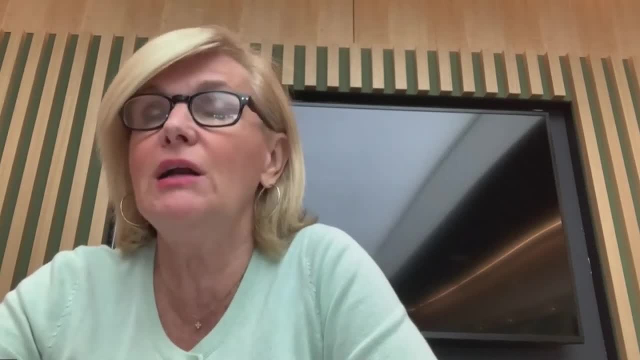 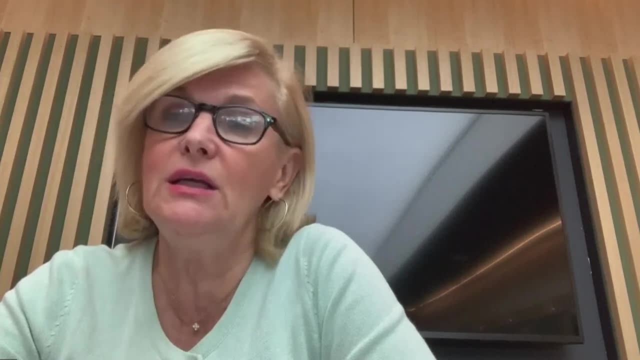 As you can imagine, being in London today at 42 degrees is so exceptional. You see that The fatigue, you see people struggling with the fatigue, you see people struggling with this condition and they are not prepared And adapted for essentially what we are concerned with in the pulpit show, in. 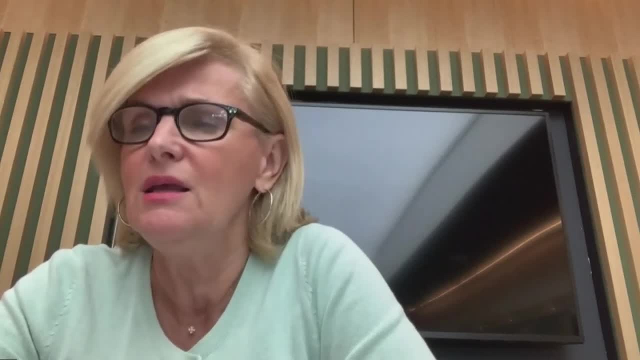 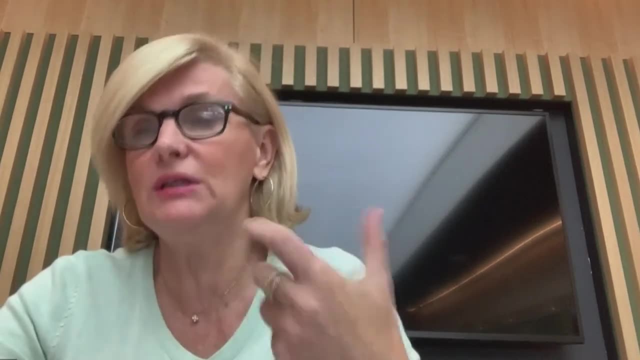 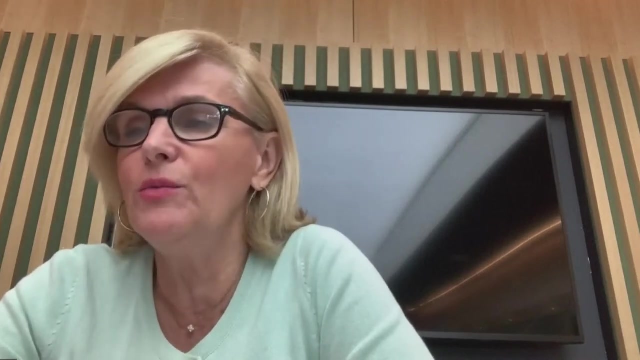 terms of this Whoa, this will be affecting human health is because of these heat will and adapted for essentially what we are concerned with in the pulpit show in terms of this will be affecting human health is because of these heat will, أو, And this can result in a cascade of illnesses. And this can result in a cascade of illnesses: dollar, dollar cramps or a heat exhaustion or heat stroke, hyperthermia and, of course, changing on behavior. You will have a very strong impact as well. We are seeing more and more on mental health or certain. 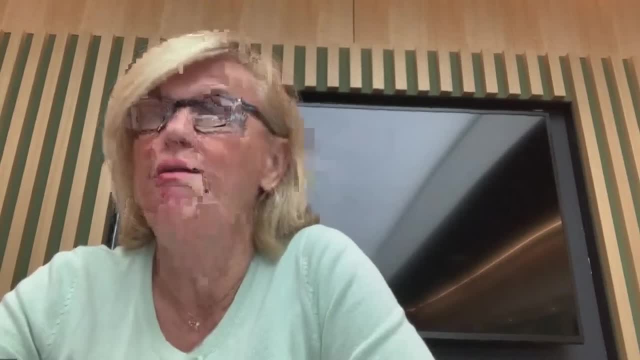 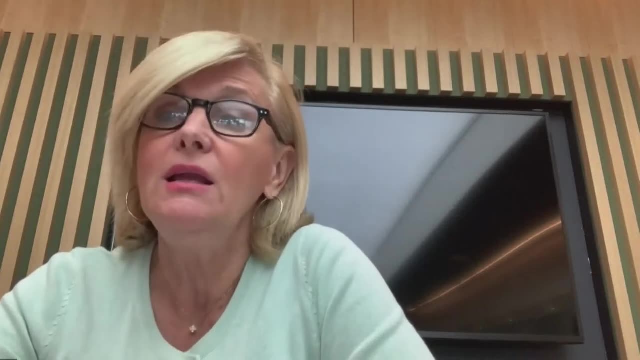 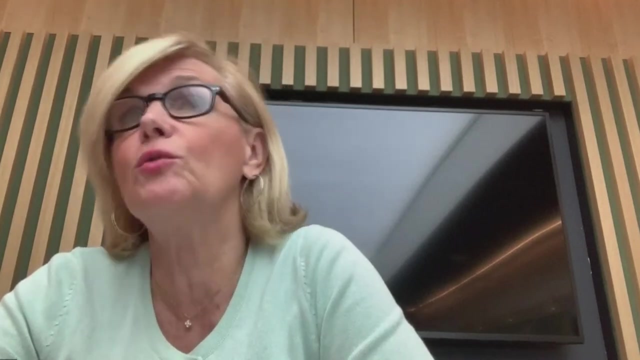 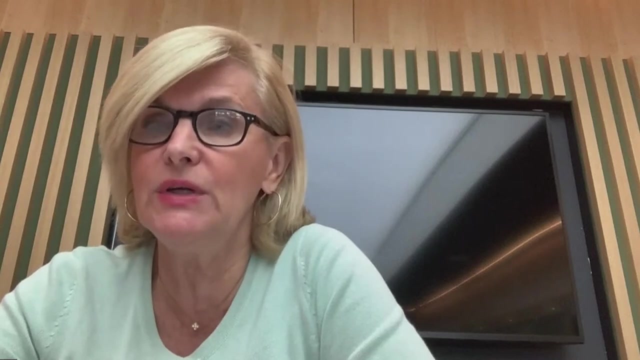 aspects that people will be feel very much affected by this heat and not having the capacity to sleep properly. In addition to that, obviously, people with previous chronic conditions, kidney conditions or people working outdoor. we are very much concerned about the workers outdoor being exposed to very high temperatures and maybe without the adequate equipment or preparation to 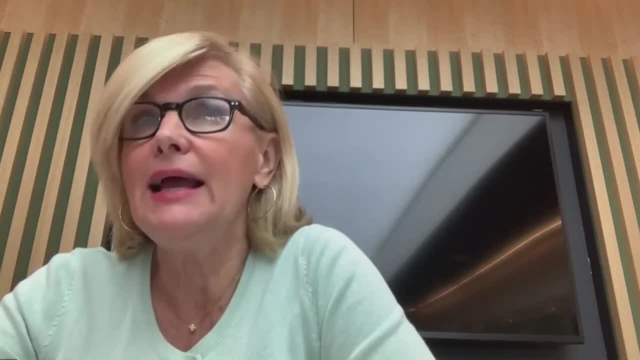 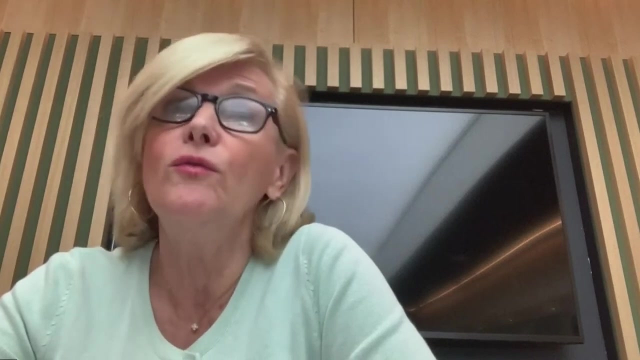 cope with that. As you can imagine as well, the health system will be challenged by this. what could be an increase in the number of people going to look for health facilities and health assistance, and that will be compromising as well. Of course, you can imagine that accidents can occur more often. 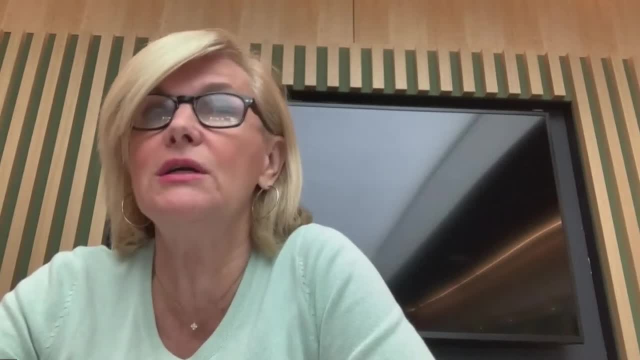 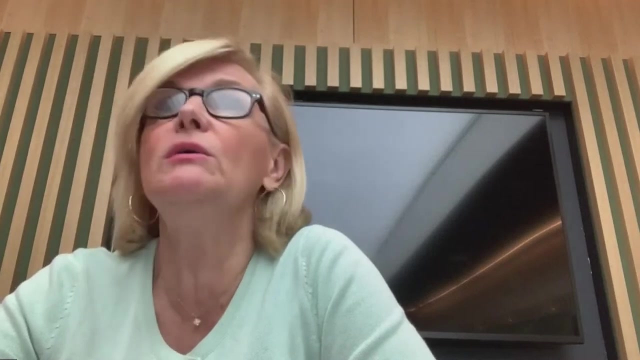 particularly in terms of occupational workers- I mean on the working environment, because you have less attention, you have more fatigue, you have exhaustion and you don't have the same capacity to react that you will have in normal conditions. The most vulnerable will be obviously the people with previous chronic conditions. 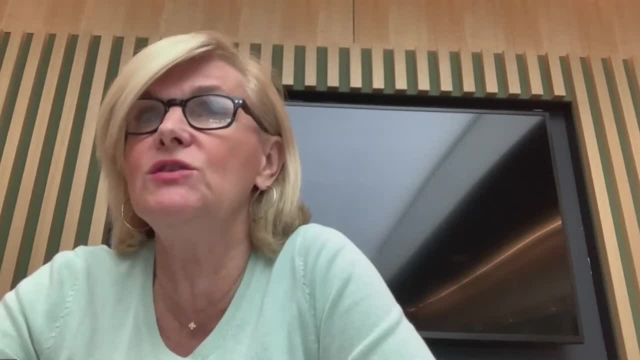 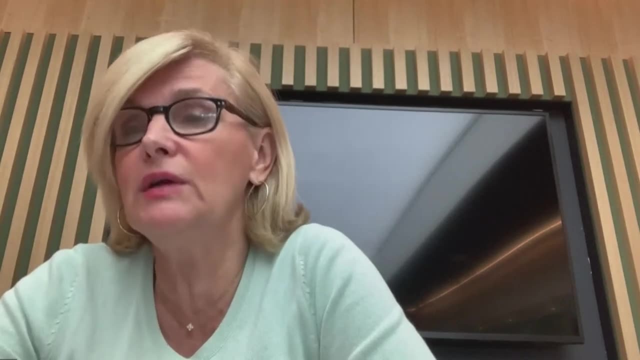 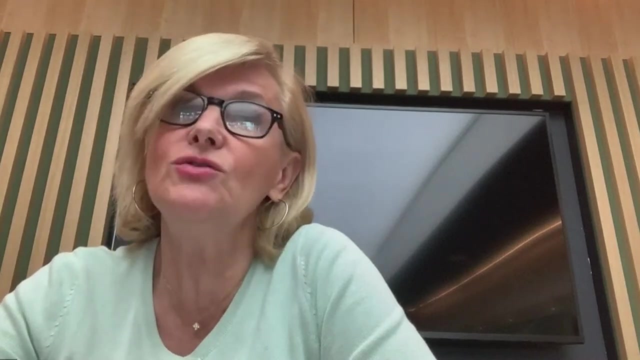 old people and very young people as well, children and pregnant women. That's why the recommendations are very logical: We want people to, whenever it's possible, to stay in a cool environment. If you cannot have a cool environment, make sure that you don't have physical activity. 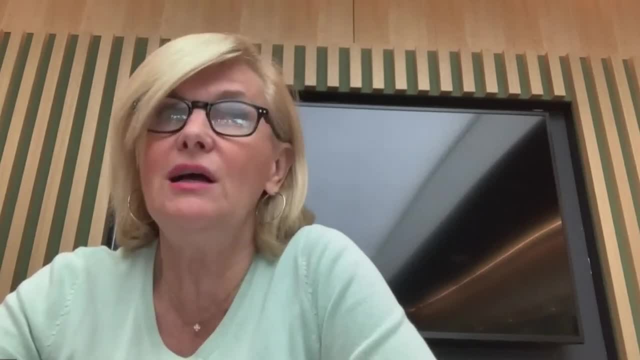 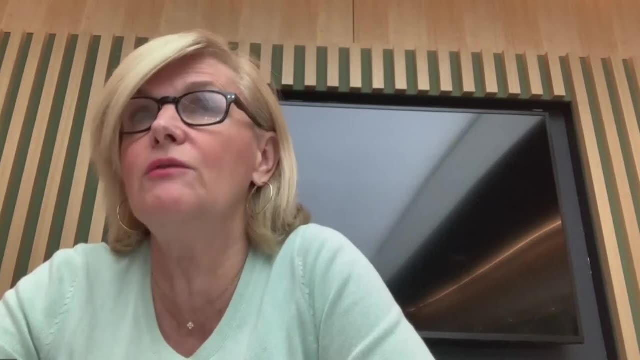 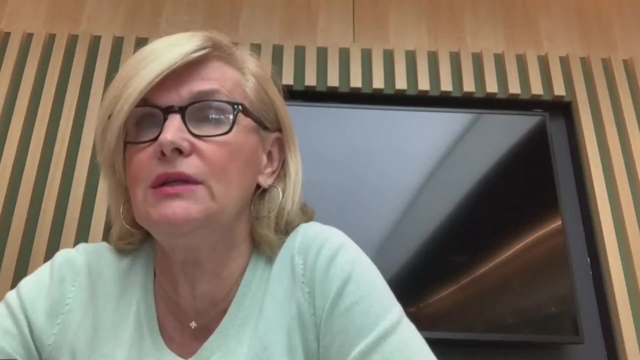 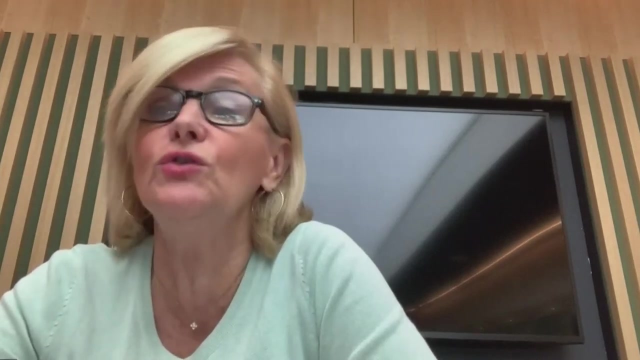 very intense. You keep very much hydrating yourself. Obviously, do not exercise and protect yourself with adequate clothes And, if you can afford that, go into a place where you can have air conditioning for at least a couple of hours a day, Avoiding and having shadows whenever it's possible and making sure that you don't drink. 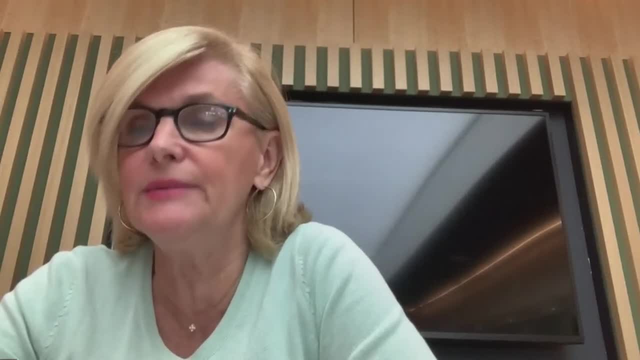 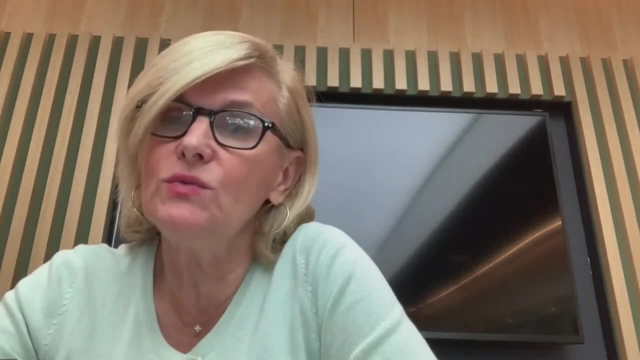 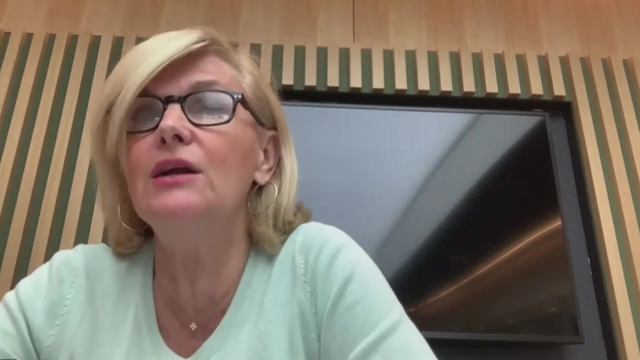 alcohol, because that will accelerate. The other thing that we are very much concerned is that when this heat wave coincide as well with high levels of pollution and therefore that will exacerbate the respiratory, cardiovascular in general diseases and condition, And this is a major concern as well for for those. 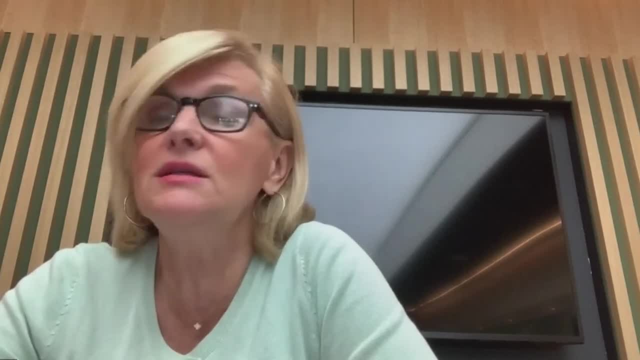 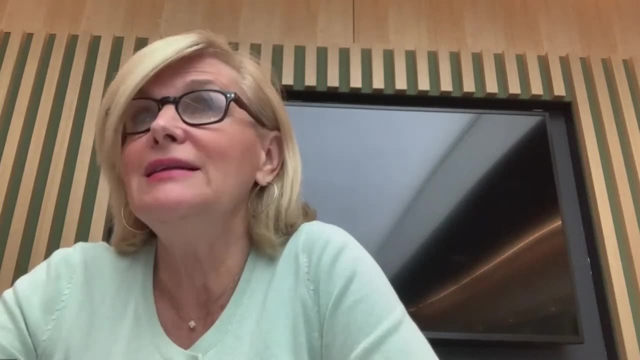 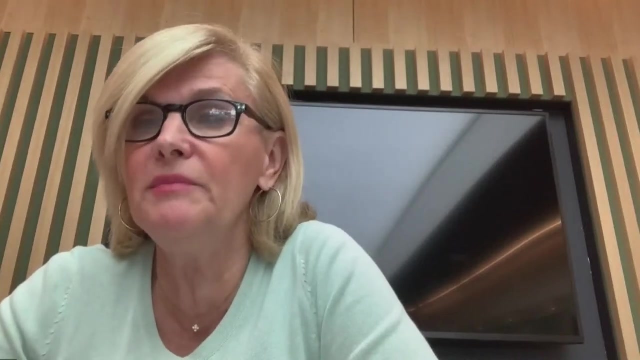 big urban spaces where the cities are not well adapted to cope with these high temperatures. Of course, the best solution to this will be again being very ambitious on tackling the causes of this global warming. We have been alerting for a long time that climate. 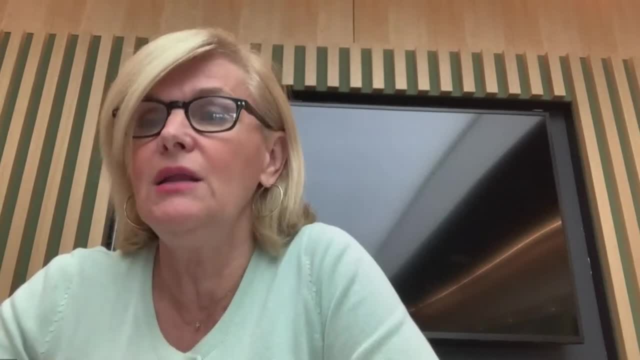 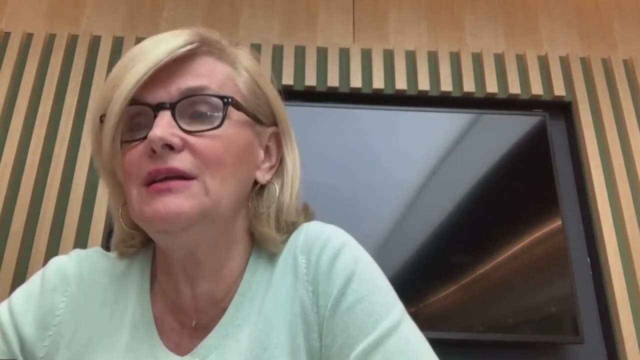 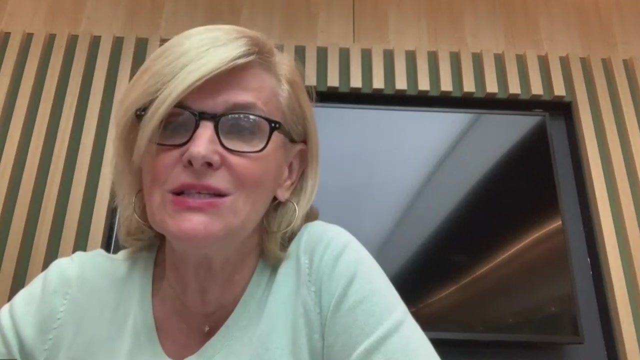 change is affecting very much human health and therefore taking measures to reach the zero carbon and accelerating the transition to clean, renewable sources of energy, Stopping this whenever possible and as quick as possible. The acceleration to renewable sources of energy non-polluting. 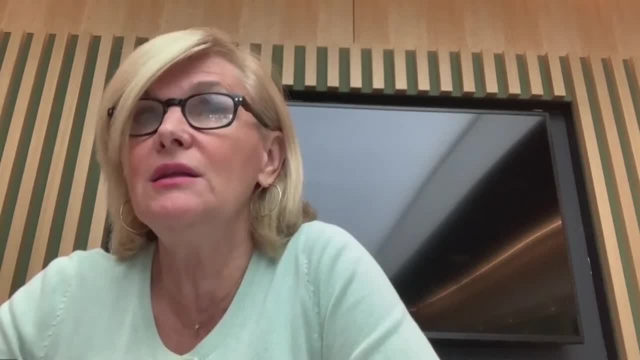 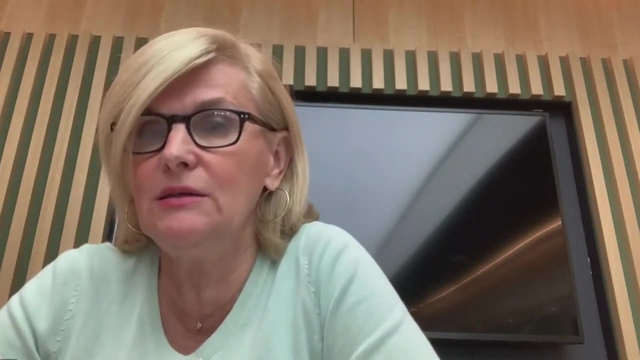 sources of energy will be extremely important. I think this is a good call for all of us that there is a need to tackle the causes of climate change, that we have been alerting the scientific community and many others have been alerting for a long time that this is. 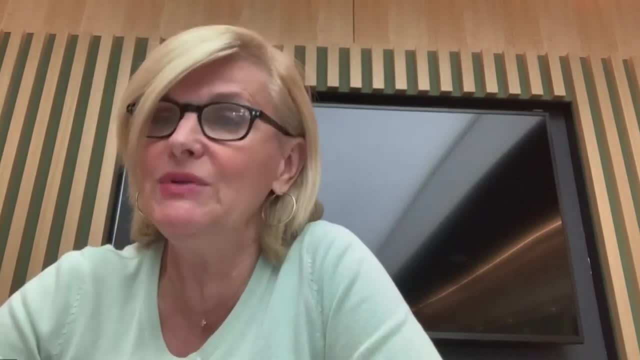 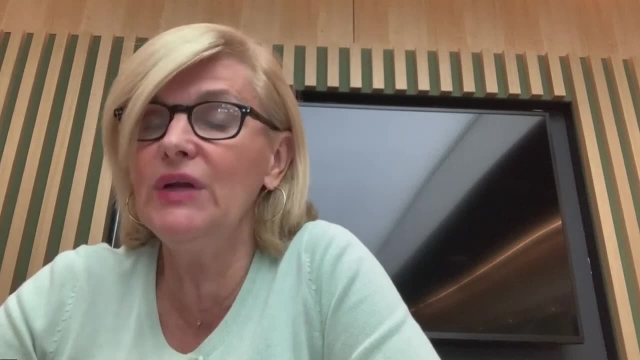 extremely important. So I hope that not only we will adapt and prepare our cities to cope with the heat waves that are becoming more and more frequent. There is a figure that is very dramatic but we need to put on the table in 2003,. 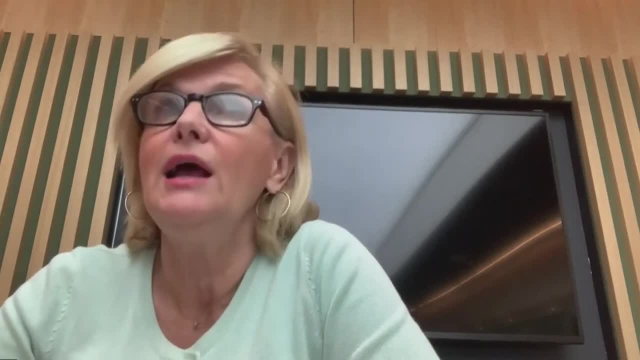 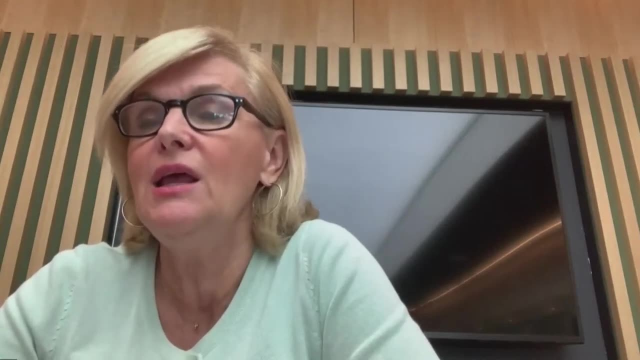 only in Europe, we have- as mentioned already by Professor Talla- 70,000 deaths, and now we know that the number of people exposed to heat waves is increasing. only in 2017, it's increasing by 125 million people more exposed to these heat waves. So again, adaptation. 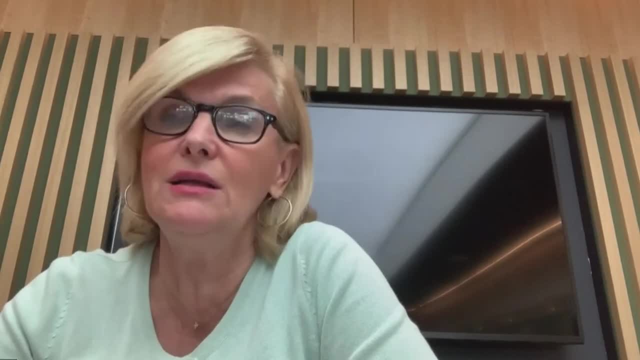 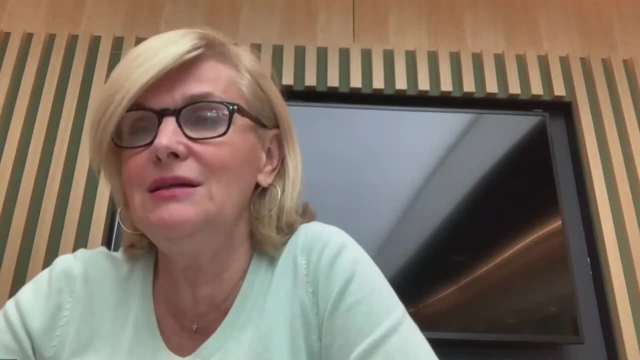 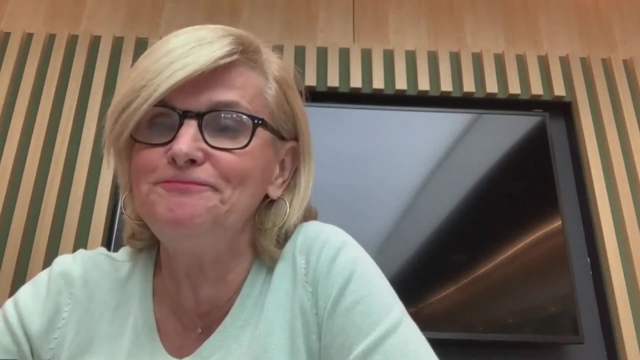 I think we need to get there And I know that we are struggling with another problem and we have to try to do something that is to do with this problem. So, yes, we always have to do everything we can to fight this and to tackle the causes of climate change. 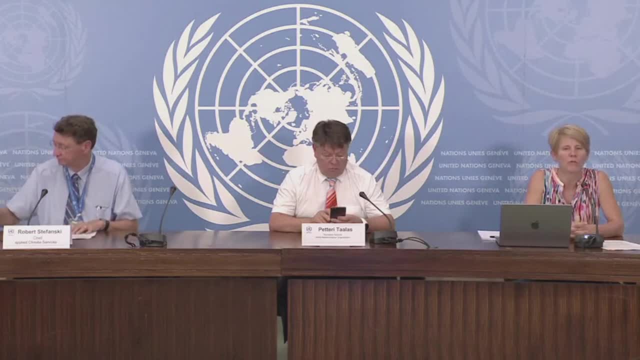 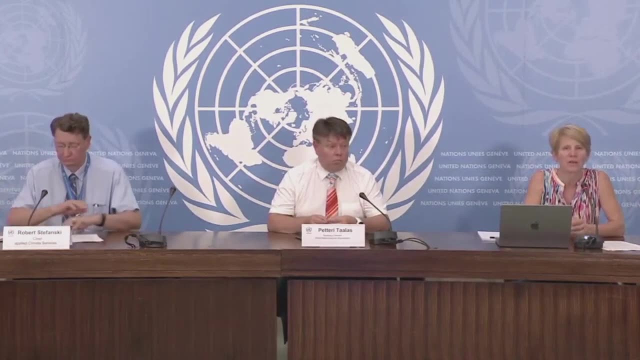 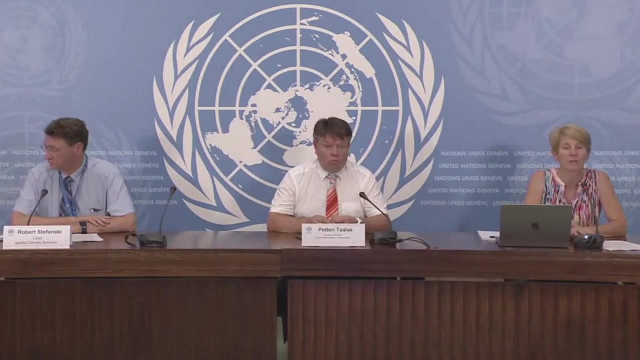 Thank you Over. Thank you very much, Maria, and now we will open the floor to questions Callas in priority, because he will have to move back to the office for a live interview for the BBC very soon, And then we will take questions for the other two experts. 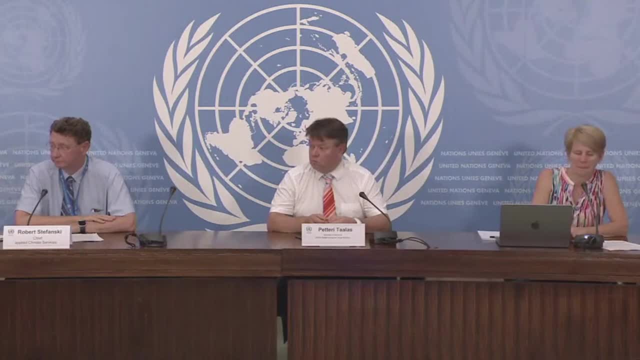 Yes, Christophe. Christophe Vogt, Agence France-Presse. Thanks for taking my question. You were talking about, or you have been talking about, the effects of climate change for quite a while now, telling people that this is going to be dangerous, that the temperatures are going to go up. 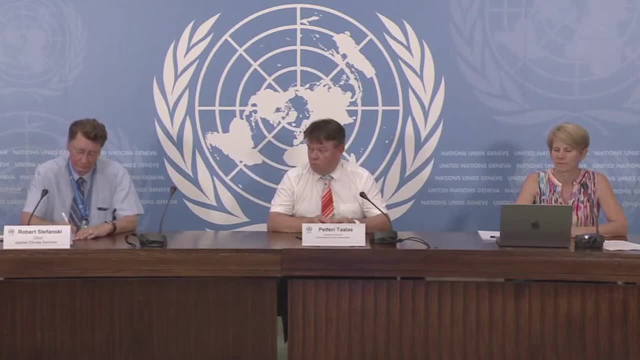 I remember many press conferences like that. Do you think that this heat wave, this effect, is now finally going, the one that is going to change the minds? And second, the second question is: what can we do to mitigate, Like telling us that you know this will not go down before 2060.. 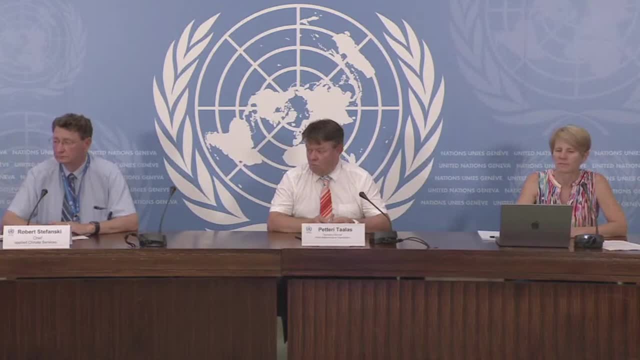 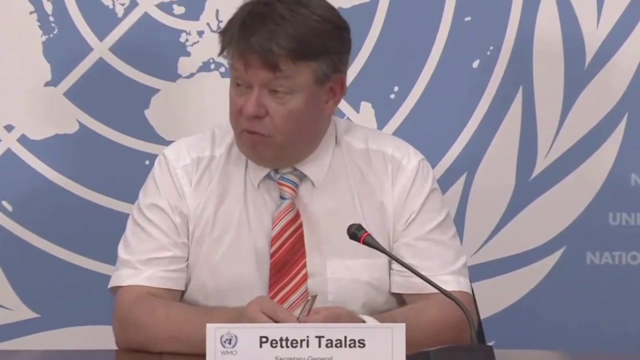 I understand that scientifically it's important, but on the other hand it doesn't give us much hope. So what can we do to mitigate individually, but also on a larger scale? Thank you, Yes, So, as I said, these kind of events, they are becoming more frequent and this negative trend will continue for the coming decades. 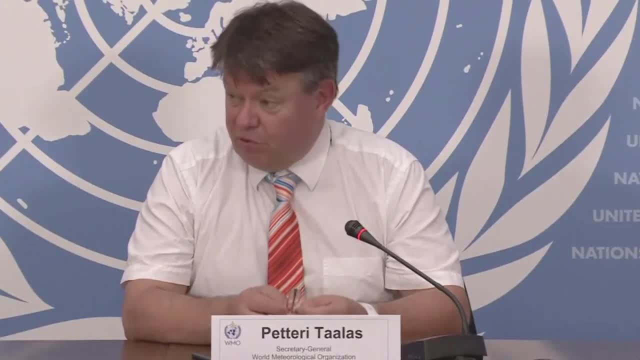 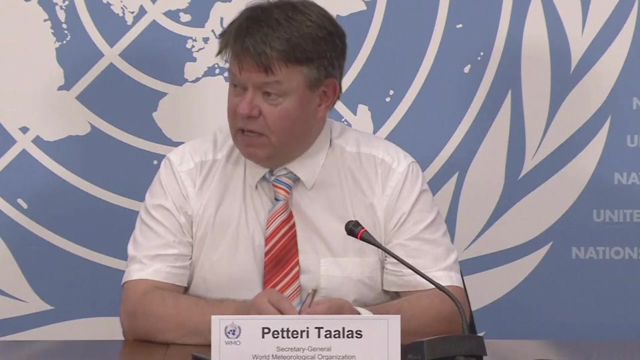 And And, of course, we have to adapt to climate change. That's also very, very important, And we have to make sure that we have enough facilities where people can stay in colder, cooler conditions, And since this 2003 heat wave, many countries have improved such facilities. 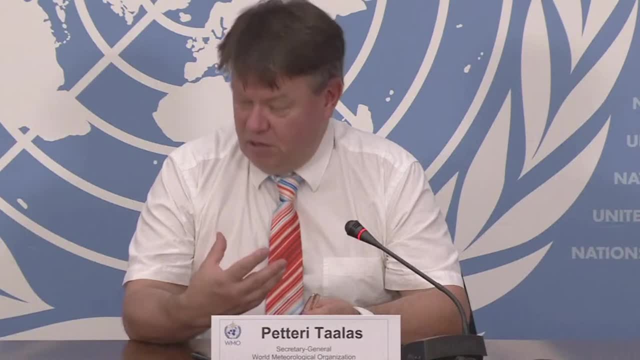 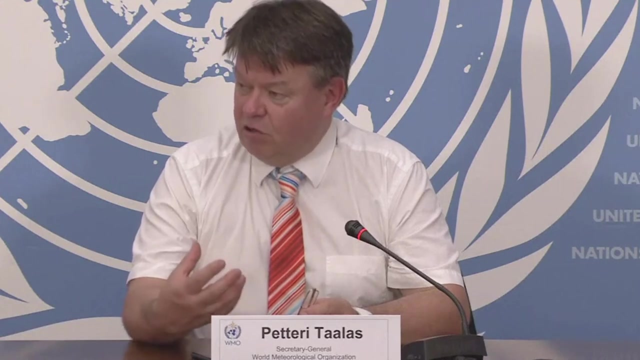 And also we know more about the health risks related to this, So we have better means to mitigate. but of course, because these events are becoming more frequent, this problem will be also worse in the coming decades And we will not be able to return to the current or the previous climate. 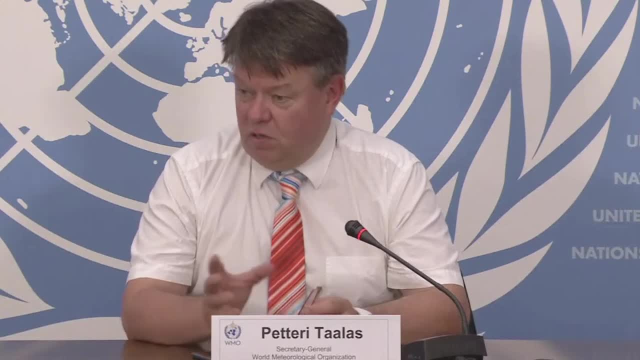 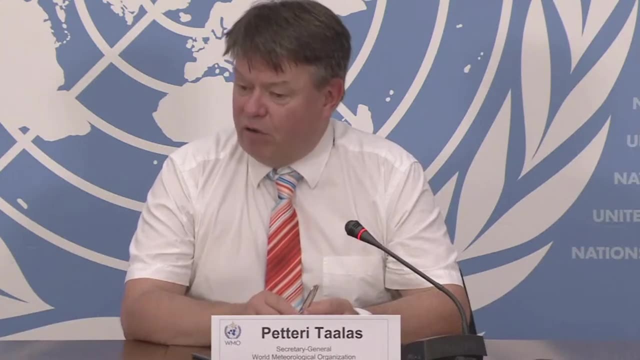 And at the moment, we are heading towards something like 2.5 degrees warming, And that means that we would have much higher Amount of these kind of events in the in the future as part of our normal, normal climate And and and these kind of events have been also wake up calls for human beings. 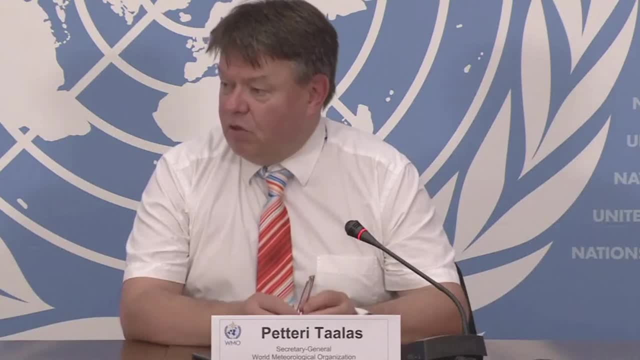 Once meteorology community started talking about climate change, especially in the eighties when we started establishing IPCC, it was seen as something theoretical And most people didn't believe in. in In our scenarios, which have been, which have, we have been able to demonstrate that they have, they have, they're now taking place. 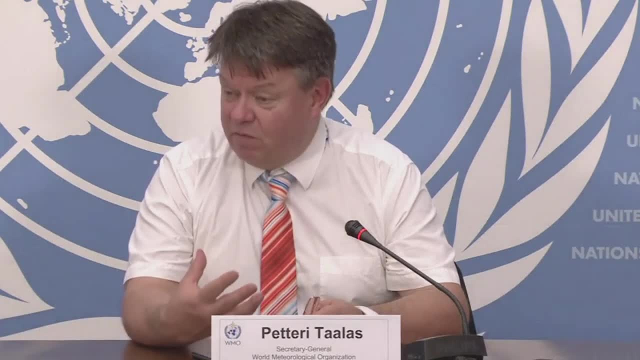 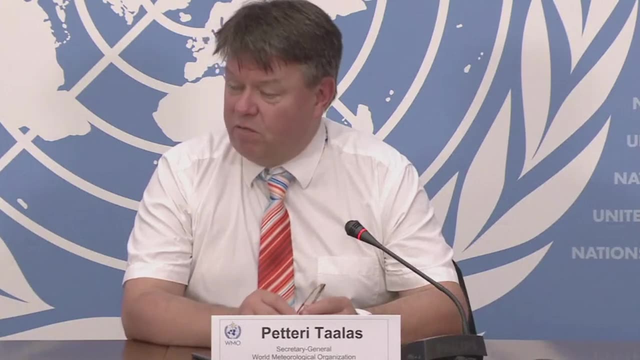 And the fact that we have started seeing impacts of climate change worldwide. that has been a wake up call for decision makers and growing also for the private sector companies. So this awareness is much higher than it used to be And and and. luckily, we have also better means to mitigate. 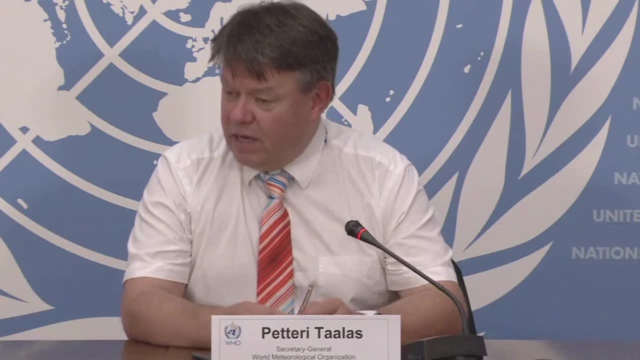 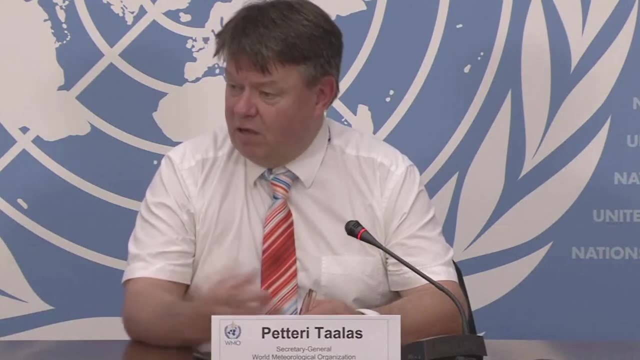 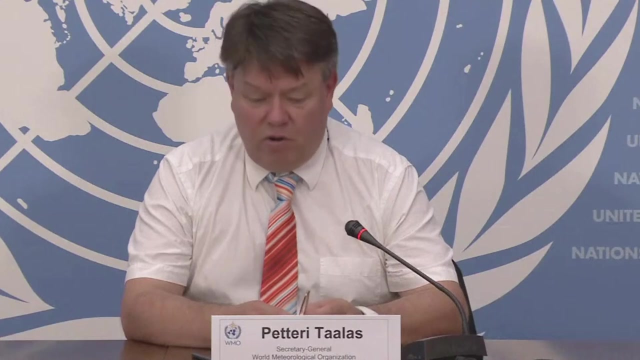 It was demonstrated That we have in energy sector a good means for for climate friendly solutions in transport means we are going to have more and more such means available And and also in our everyday diet we can favor. favor more vegetarian diet, for example. 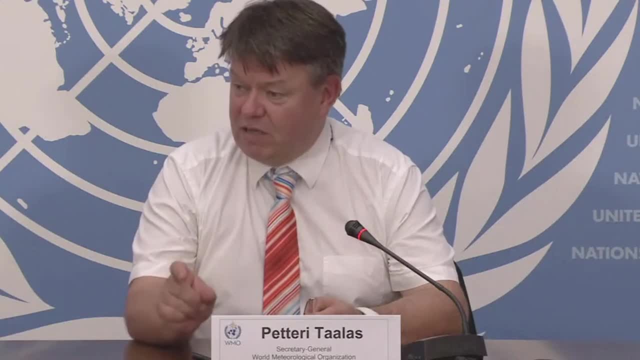 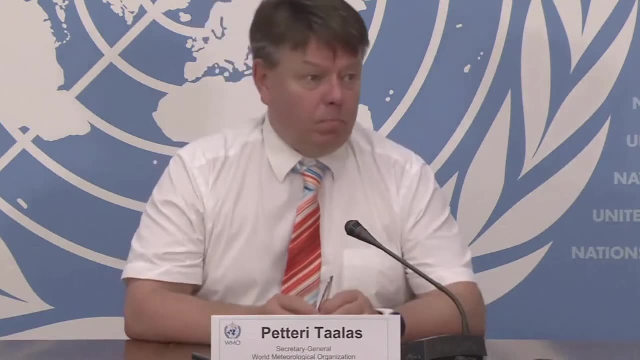 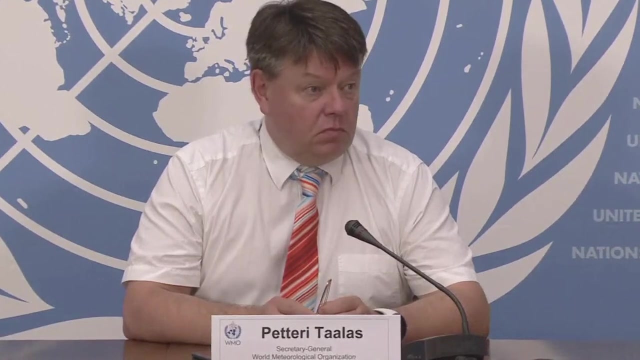 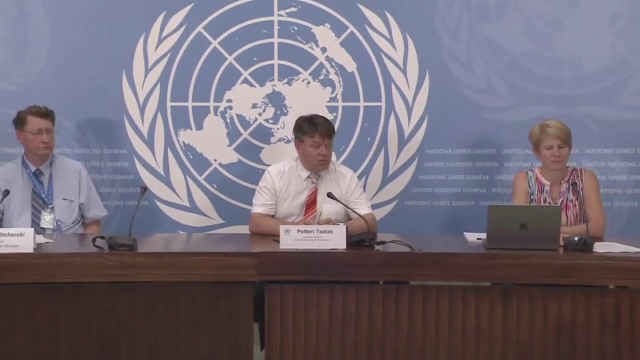 So so the means to solve this problem and also the price is related to this mitigation. They're getting getting lower. Thank you very much. Any other question in the room? Yes, please? Thank you. Our global TV in Brazil and Brazil is now suffering with high temperatures. even it's winter there. 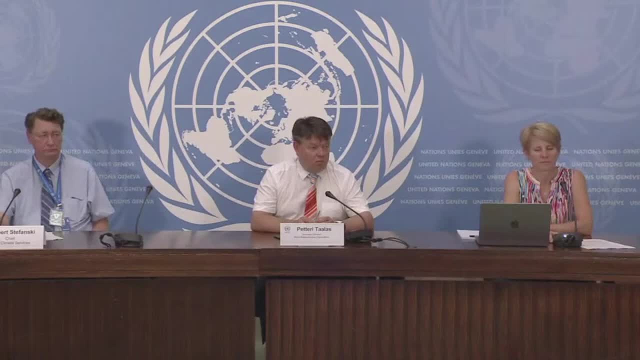 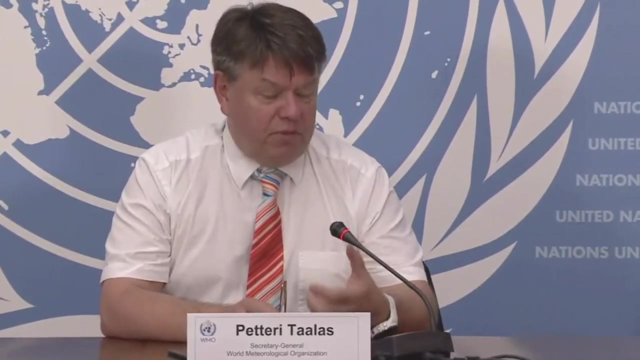 So could you make a relation between the extreme weather in Brazil here and climate change? Yeah, We have seen. Yeah, I mean this global climate change which has had an impact on global temperatures, on global reputation, patterns and melting of glaciers and sea level rise. that's happening. 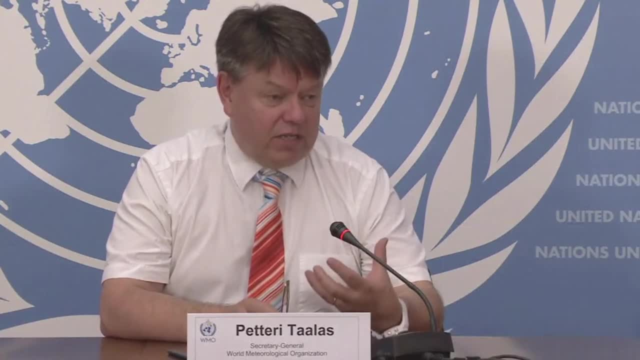 And that's also affecting Brazil. But in Brazil, besides that, you have also affected the local climate by cutting your rainforest, which has had an impact on global local rainfall conditions and humidity conditions, and also in the climate. So that's a good point. 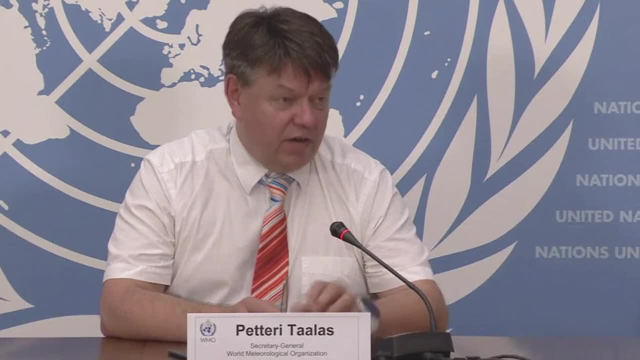 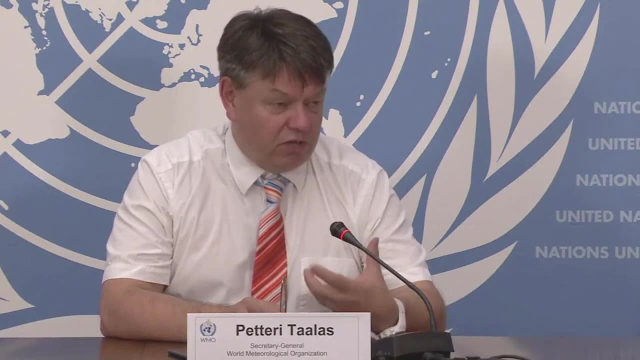 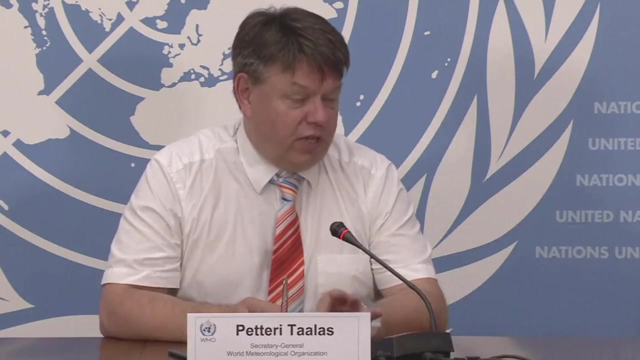 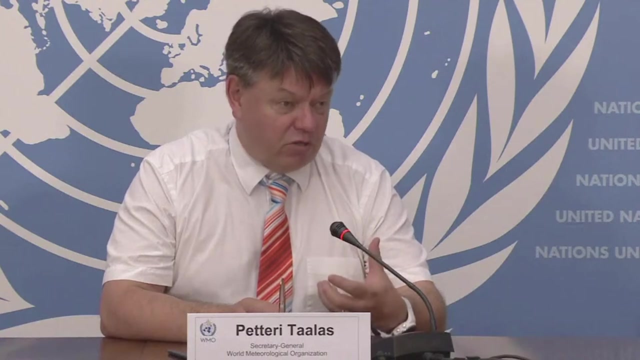 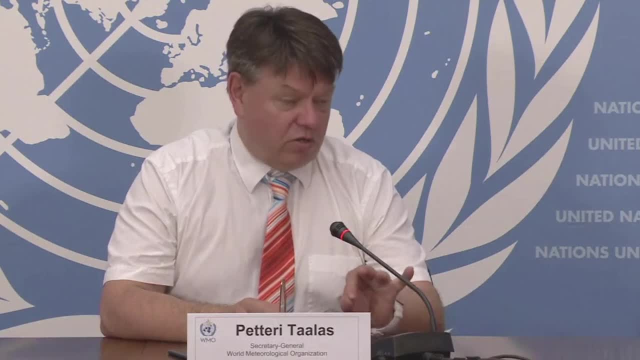 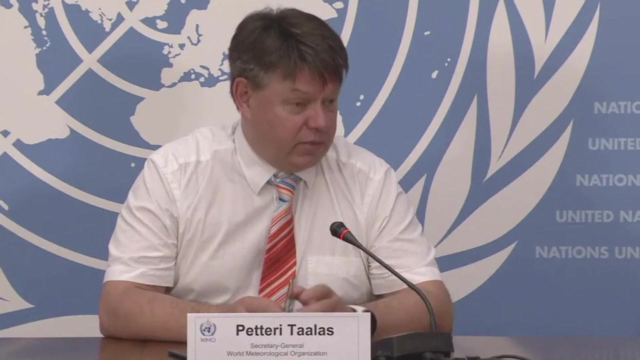 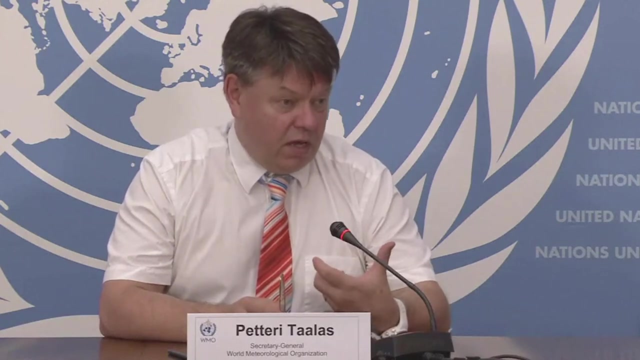 hotter and and this deforestation has also had a negative impact on the global global carbon dioxide concentrations. amazonian rainforest used to be a sink of carbon and but the most recent studies have shown that it's partly- at least partly- a source of carbon because of deforestation and- and this is also related to the diet- with this deforestation, you 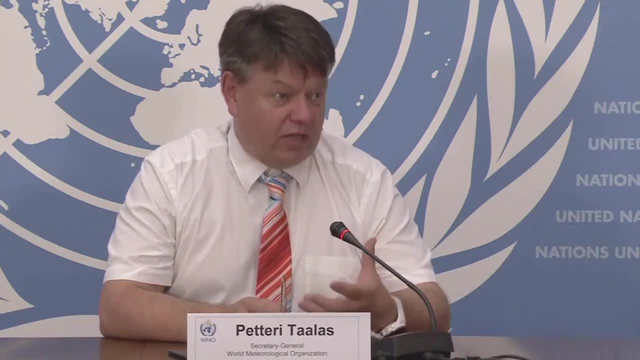 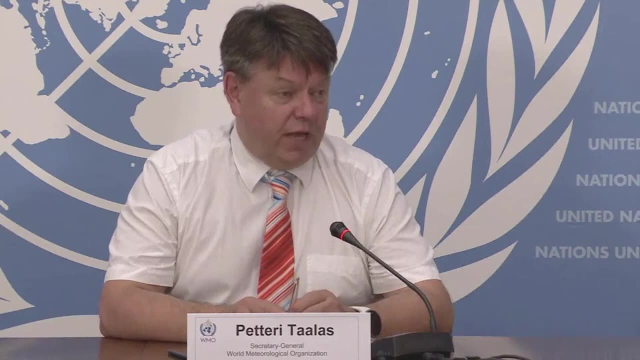 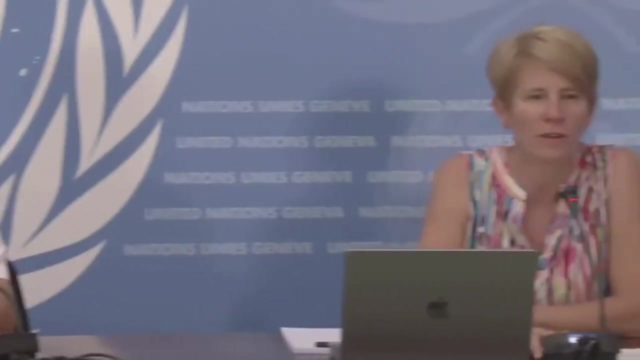 are growing, for example, more soybean for the cattle, and, and, and that's again a good reason to reduce the consumption of of of meat. thank you, and just to note that we will release on friday our state of the climate, latin america and caribbean, and you will. 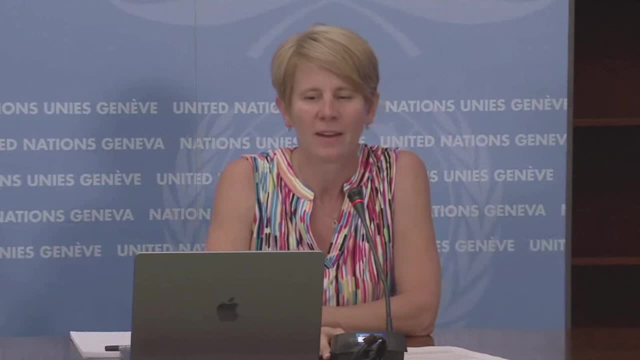 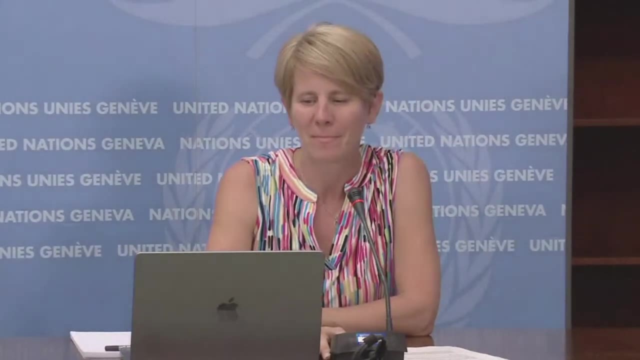 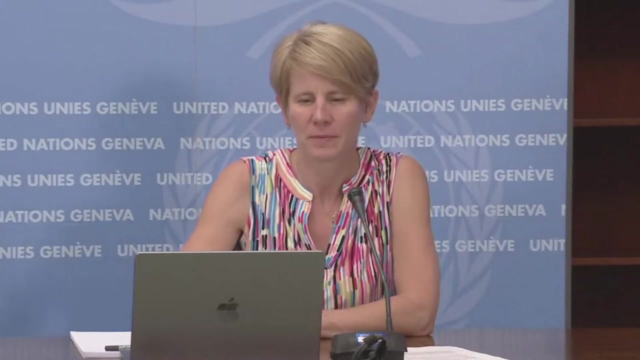 find more, more figures and statements about that. um, if no one else in the room, i want to give the floor to jamie. good afternoon, thank you very much, um, for that abrigid um wanted to um, professor, tell us. i just wanted to follow up on what you said earlier and about what, uh, christophe also. 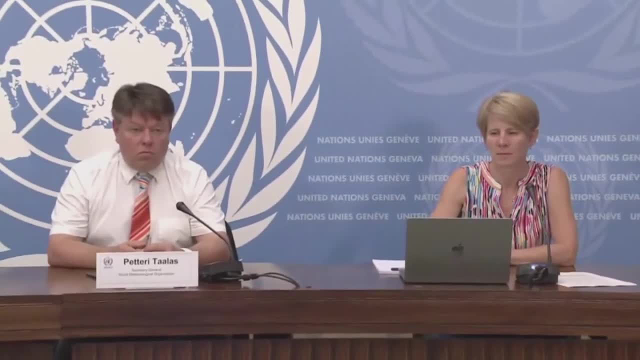 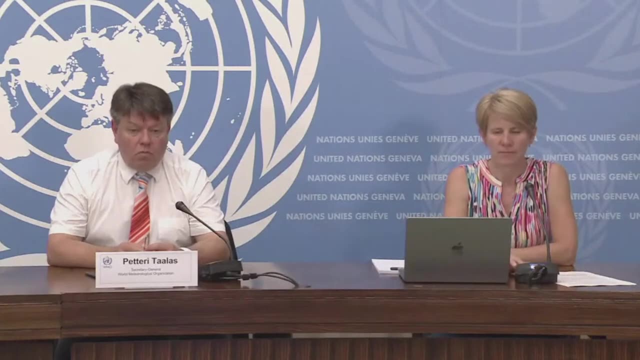 said about the heat that the climate had been in for the past two or three years. so, um, i'm very grateful to look back at the past two or three years and i can't remember exactly what you said, but i'm very proud of what you said earlier. um, you said that these kinds of heat waves are 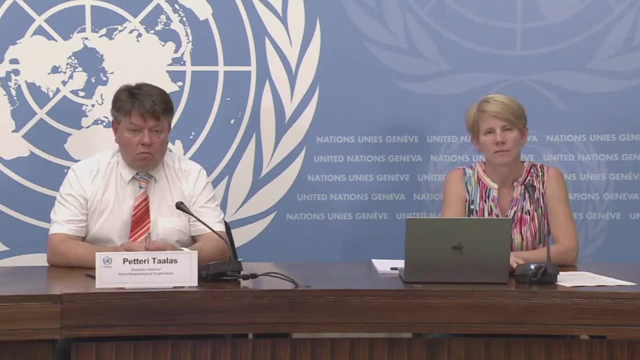 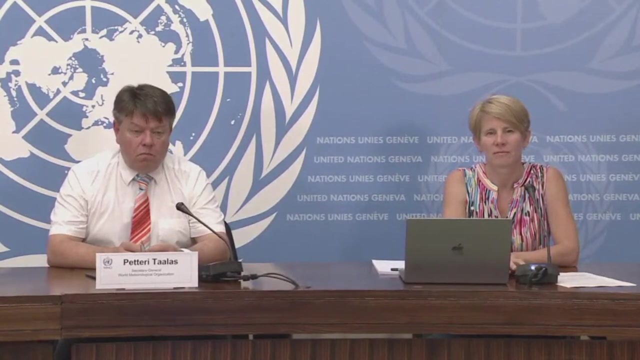 becoming are becoming more, more frequent in the coming decades and the negative trend in climate will continue. what does that mean exactly? i mean you mentioned that, that last year there was a, a trend, and just um, if i could also follow up on the 2060 forecast, is that new that you expect that? 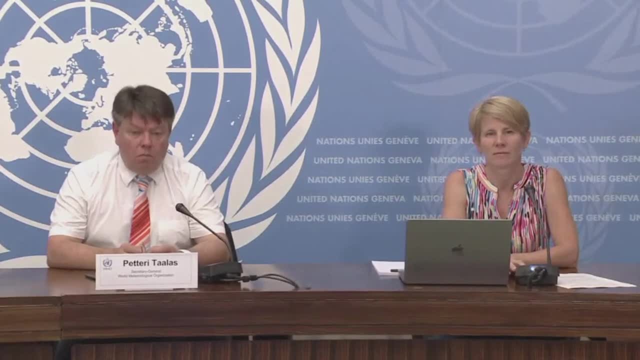 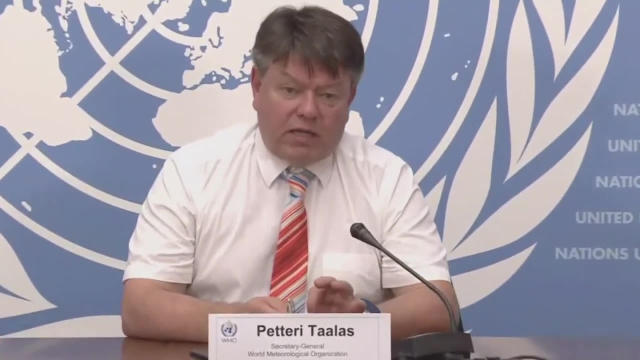 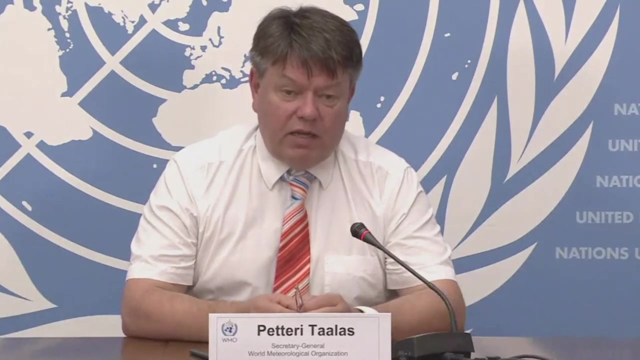 it's going to go until 2060 or is that based on new data that are old data that you've had? thank you so much. sorry. thanks to climate change, we have started seeing, uh, we have. we have started breaking records nationally and also also regionally, and and and. for example, last year we broke. 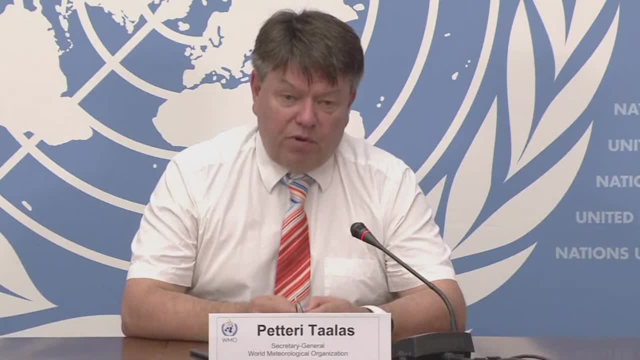 all-time high in in in europe, but we also broke all-time highs in spain, turkey and canada thanks to the impacts of climate change. of course, we will see also this natural variability, which means that we are not going to break records year by year in a single country or 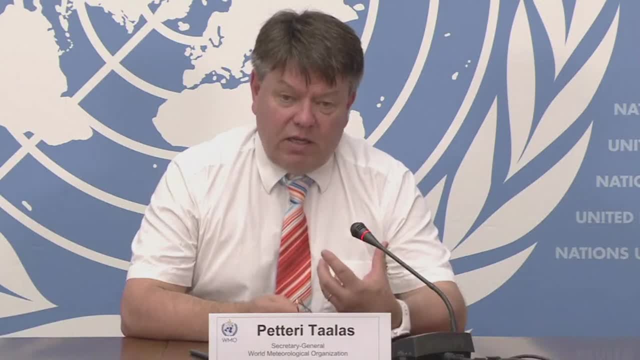 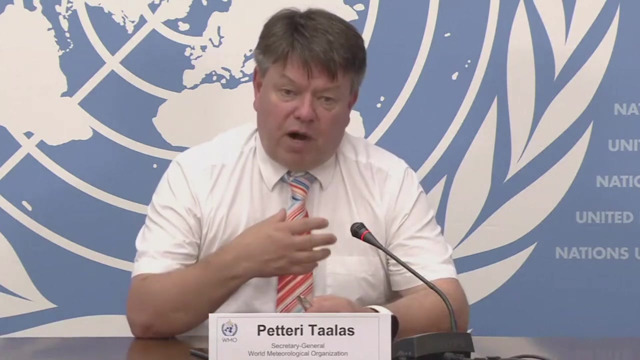 in the future, or single region. but the direction is clear and in the future these kind of heat waves are going to be normal and we will see even stronger extremes. We have already pumped so much carbon dioxide to the atmosphere that the negative trend will continue for the 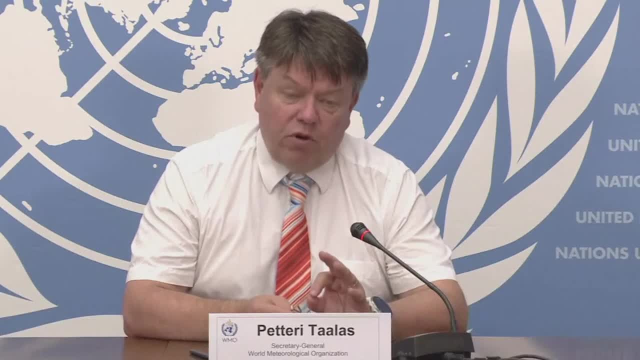 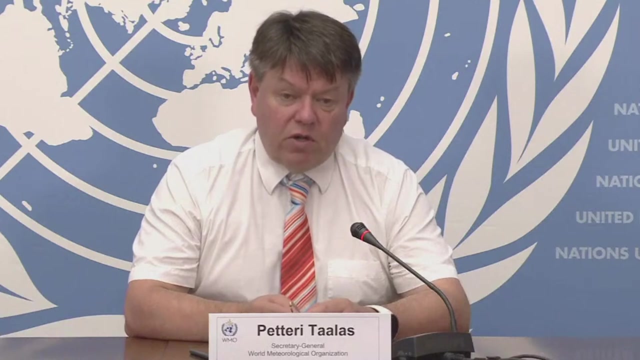 coming decades and so far we haven't been able to reduce our emissions globally. We have seen regionally good progress. for example, European countries- United States, Japan, Singapore- have been able to reduce their emissions during the past 15 years, whereas in Asian countries. 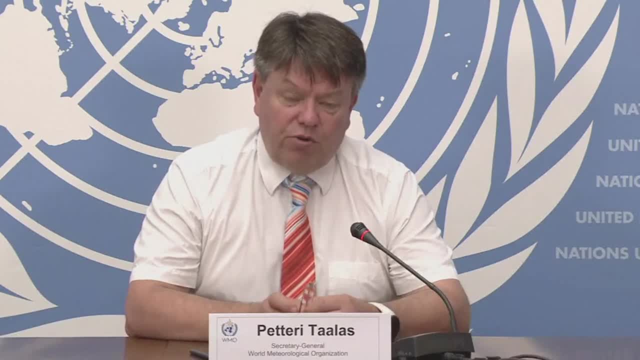 we see this negative trend continued and emissions are still still growing and therefore we haven't it's not sure that we would see the peak in 2060s if we are not able to bend this emission growth development, especially in in the big Asian countries, which are the largest emitters today. And what was the 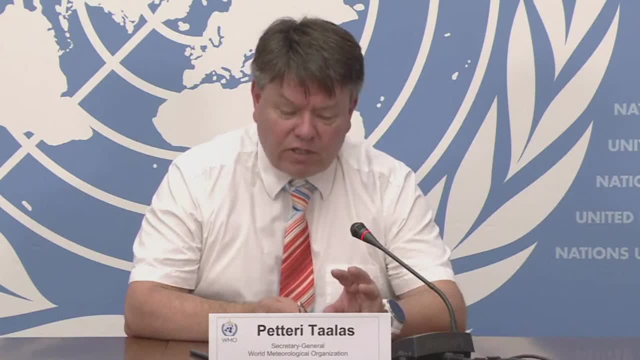 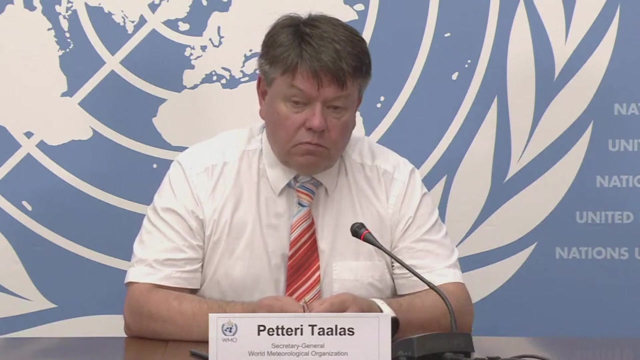 other part of the question. Could you repeat the other part of your question? I forgot that. I think it was the second part. Jamie, can you repeat the second part? Sure, yeah, it was just about the 2060 forecast. Is that based on a new data or have you known? 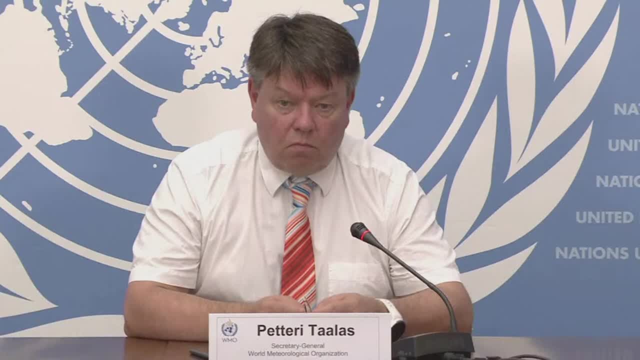 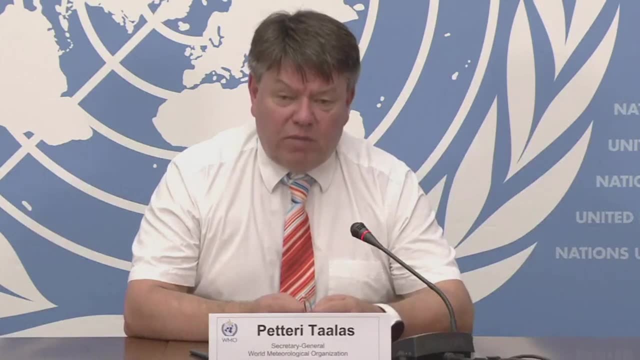 for a while that this negative trend is going to continue until then. Yeah, it has been known. of course, we were hoping that the peaking of the emissions would have taken place already, Earlier, but we have seen the reverse happening and we have started seeing a fairly rapid growth. 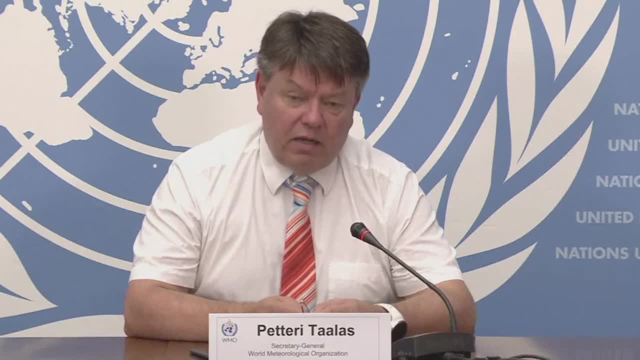 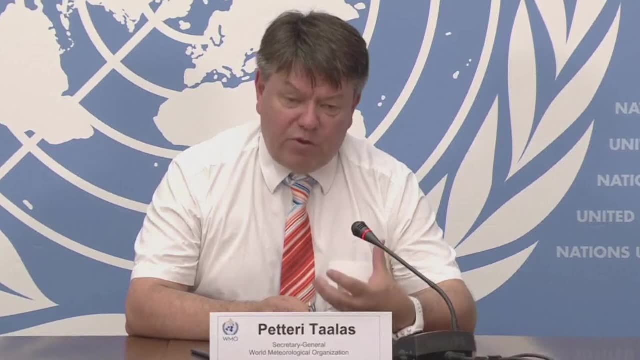 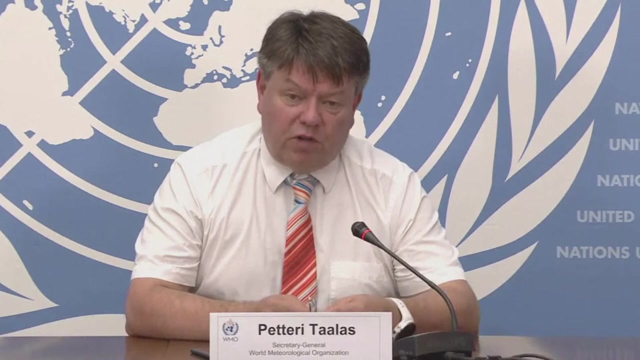 of the emissions, especially in several Asian countries recently, And we could seize this negative trend in weather patterns by mitigating. but we have already lost the game concerning melting of glaciers. so we expect that this melting of glaciers will continue for the coming hundreds of years, or even coming thousands of years, anyhow, and also sea level. 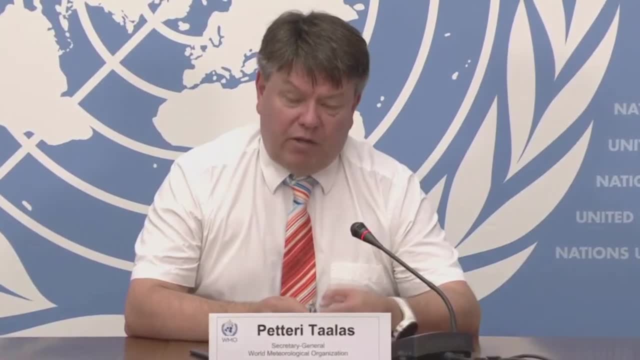 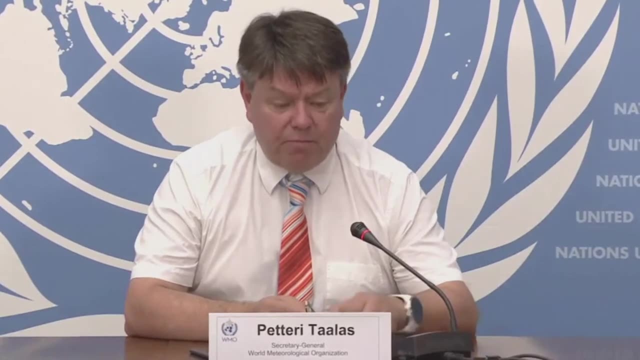 rise will continue for the same period. That's good, bad news and that's because we have already reached such a high concentration of carbon dioxide. And the reason- if I could just follow up on that part of the reason- I asked that question was: 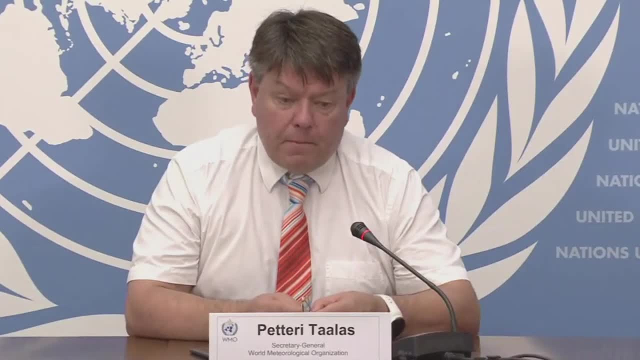 because we're seeing a number of countries going back to the use of fossil fuels. They're sort of because of the concerns about fuel shortages and whatnot. Is there any way to judge whether or not that kind of return to fossil fuels is going to have an impact? 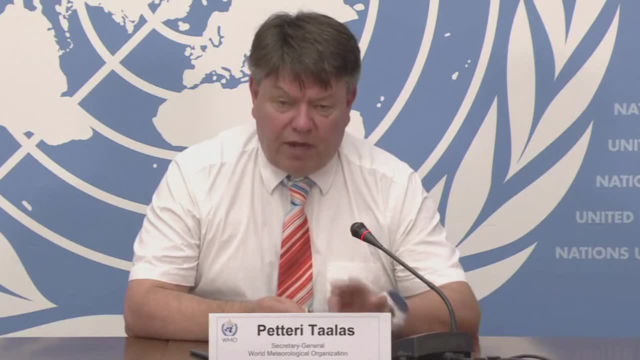 Of course, we may see two types of development in the coming years. In the short run, for example, European countries which have been highly dependent on gas import from Russia and they have to comfort their energy need somehow, and it's likely that. 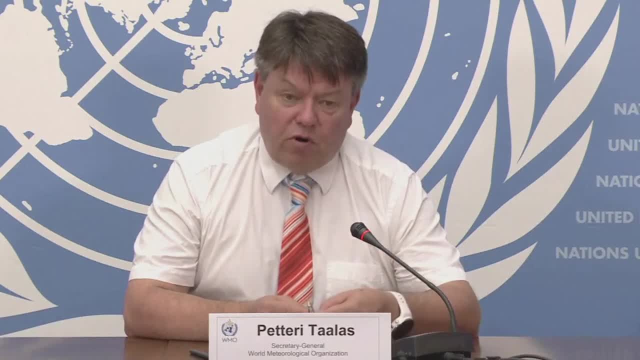 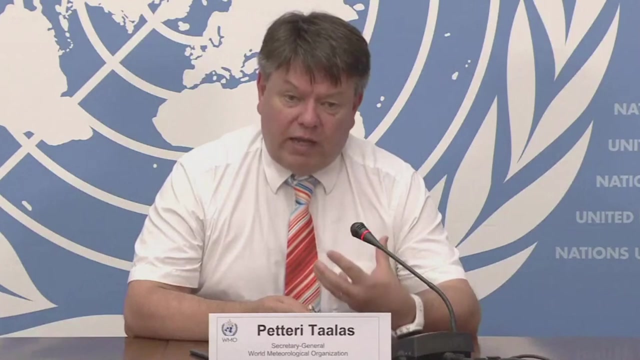 some European countries may use more coal to produce enough energy, But in the coming five to ten years there's a chance to reduce our dependence on fossil energy more and that's in a positive. that would be the positive scenario and that's also likely to happen- that we will. 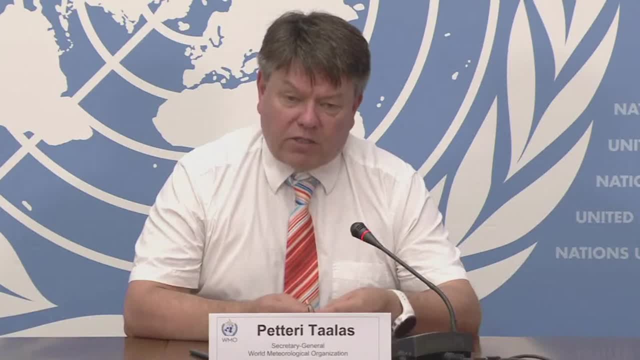 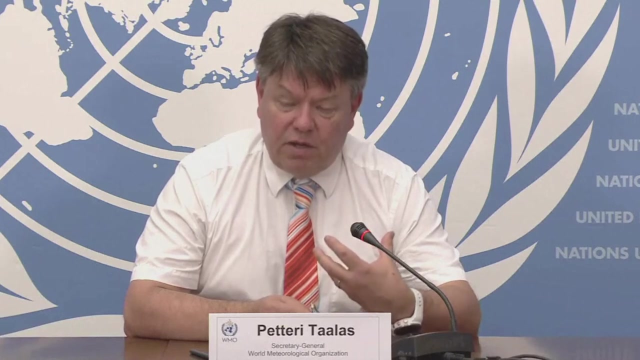 speed up reduction of use of fossil energy, at least on European scale. And since we have seen this Russia dependence and related impacts on financing of the military actions, there's a possibility to speed up climate mitigation efforts and start comforting the energy needs much more with renewable energy and also with nuclear energy, So that's likely to. 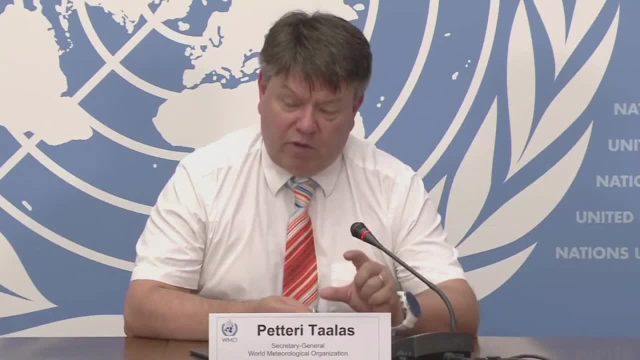 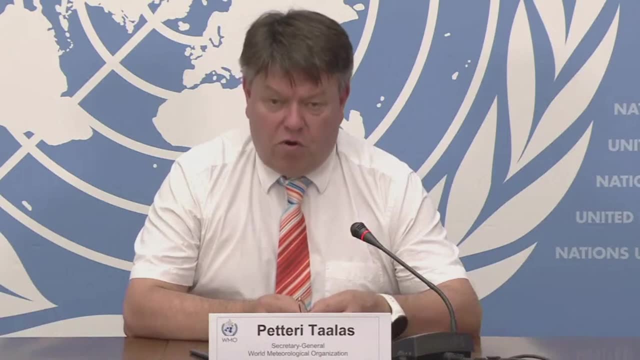 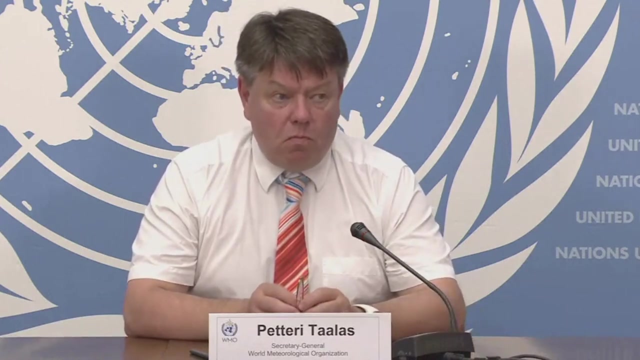 happen, at least in Europe, in the long run, five to ten years from now. But for the coming couple of years it may be that we will use more coal to comfort the energy need. Thank you, A question from Paula Dupra. 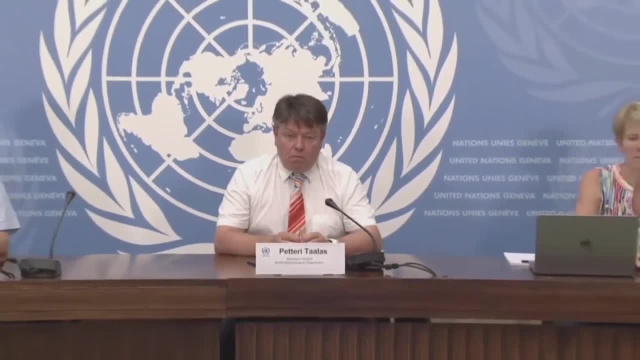 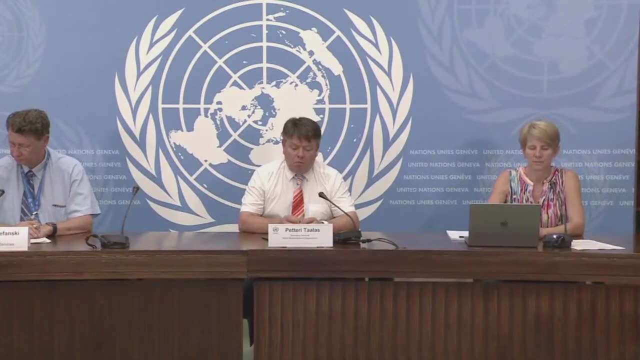 Yes, hi, thanks for taking my question. Yeah, this is for Swiss Info. My question is about the upcoming World Cup in Qatar, As we know, a big fossil fuel supplier. It's, you know. as we know, the date was shifted but there, you know, there have been issues with. 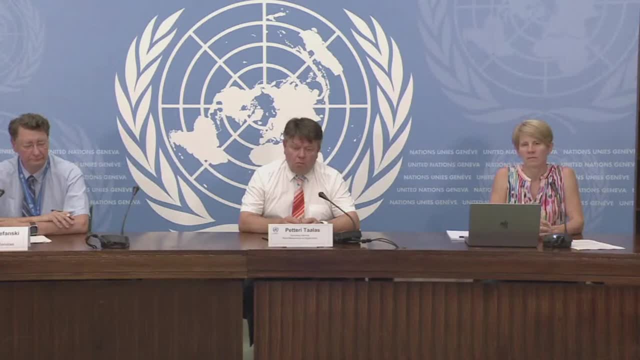 the worry about that now, about the future". So let's start and wrap up with a world cup request. also much look forward to the World Cup being held there in the middle of the summer- It's now in the Fall, but nonetheless I'd like to know. get your thoughts, Professor Tellus, on the signal. 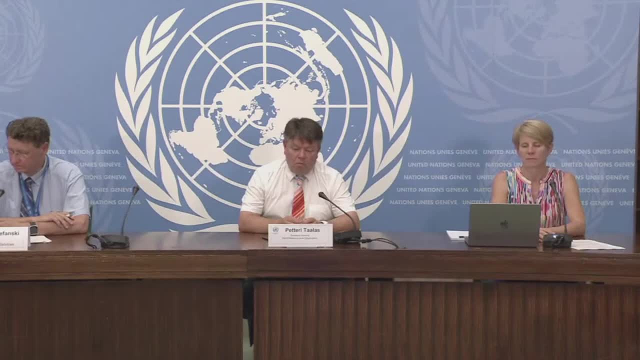 that it's a. it has already sent to the hosting this global event in a country that is active on climate change as a tool for national left to remind and we will mention. we hope that it will be here. but I'm really asked if that's okay by a government like you. I'm going to suggest get your thoughts on the Western support for global sympathetic policy on climate change for the next couple of years. 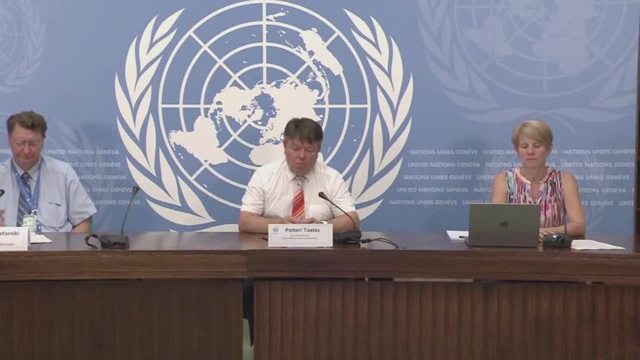 So thank you for asking me. that's great, That's great, That's great, So thank you. this global event, in a country that is supplying a huge amounts of fossil fuels that are generating, you know, this, this, this, the carbon and, of course, having a great impact on global warming. 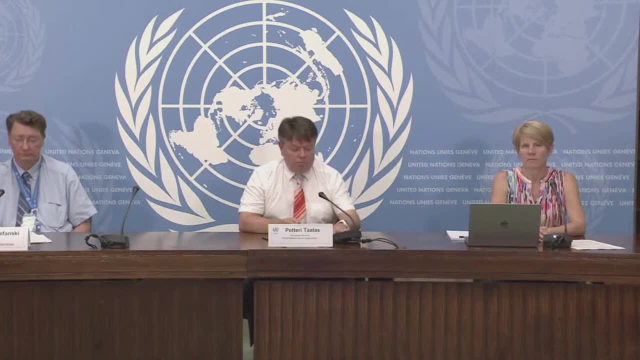 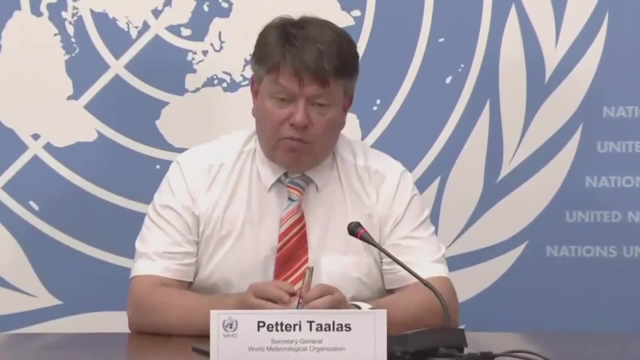 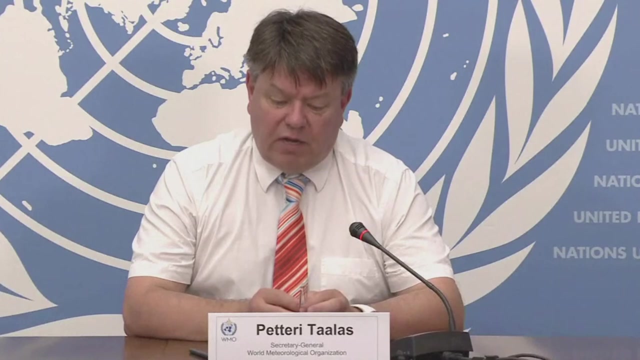 Could I? yes, could I have your thoughts on that? Yeah, of course this oil and gas producing countries. they are producing this energy for the because there's a demand of such such energy. So without the demand it wouldn't happen. 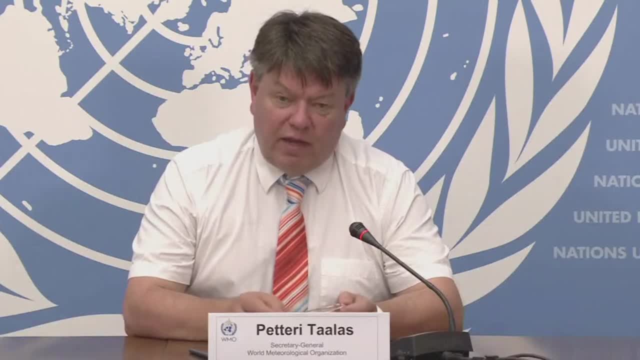 And it's it's for us who are living in rich countries. we should look at the mirror, because we are consuming those, those resources. If there wouldn't be the demand on our side, there wouldn't be market for such such sources of energy. 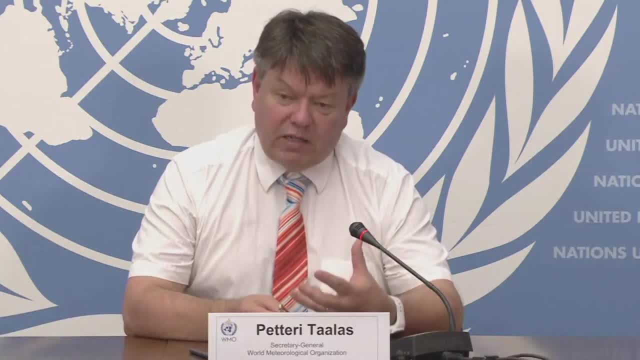 So it's not fair to blame those who are selling this kind of energy, but but we as consumers we are also responsible for for that. Of course, it's going to be a major challenge for Qatar type of countries If we seriously will reduce the consumption of fossil, fossil energy in the future. 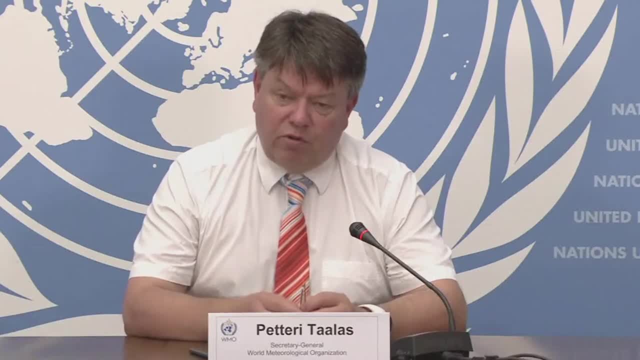 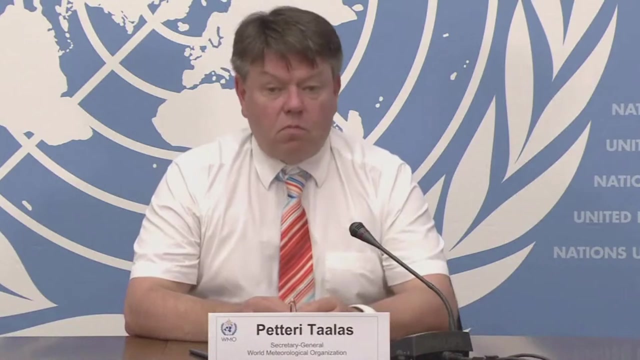 And it's a question how they will be able to carry out, keep the current standard of living there if the income of fossil energy ceases. So that's a good question, and it's not an easy question for Qatar type of countries, Gabriela Sotomayor. 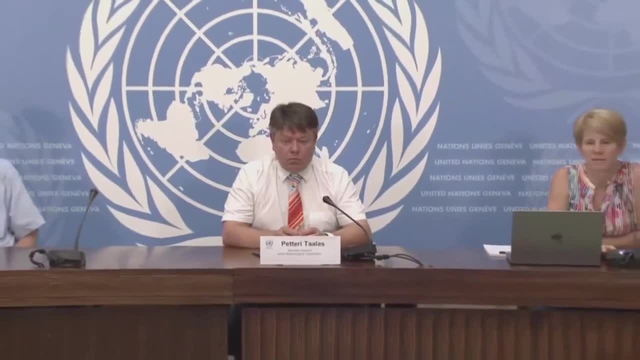 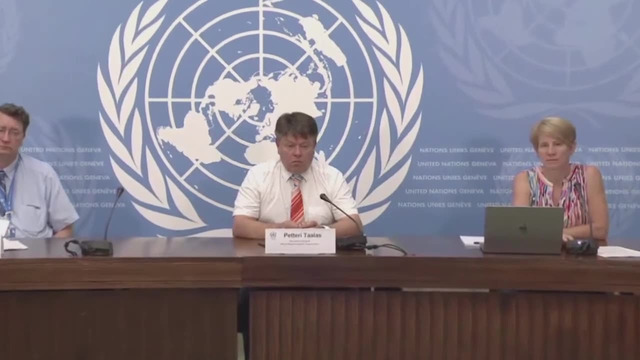 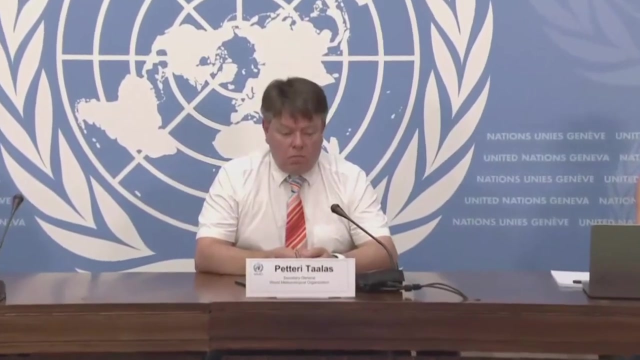 Yes, Hello. Thank you for taking my question, Professor Talas, What about the governments that seem to forget about these heat waves in the summits? Do you think that if they were in London today, they would sign the agreement? Thank you, 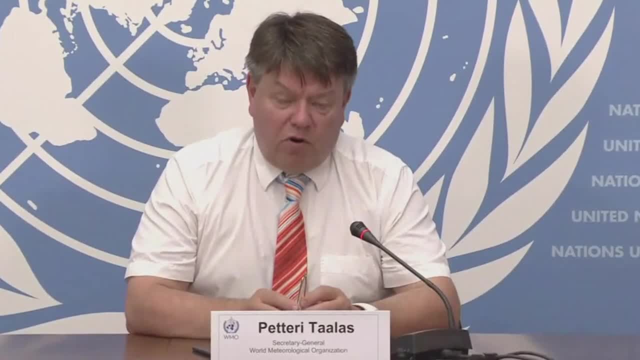 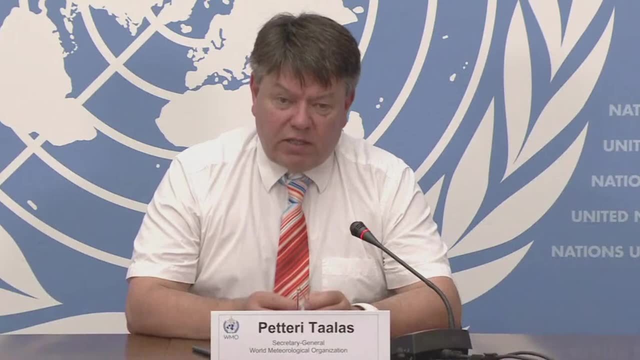 I hope that these kind of events are going to be a wake up call for many governments And I hope that also In democratic countries this kind of events will have an impact on voting behavior, and in democratic countries it's up to the governments what kind of policies they are having. 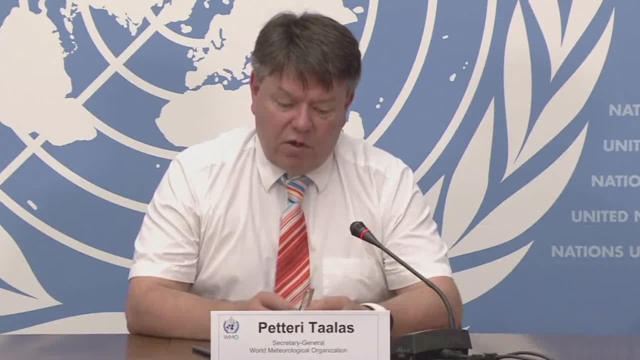 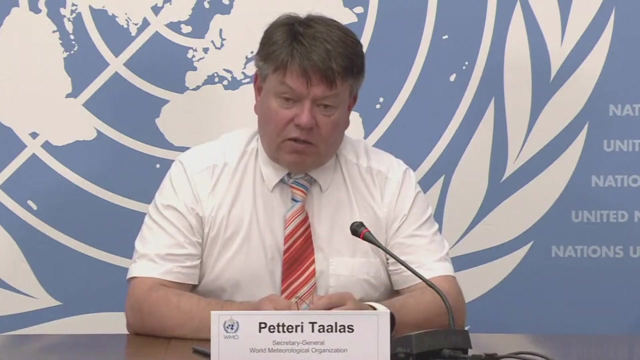 And it's also important that we have a worldwide act- and, for example, how we handle import from countries where the basis of energy is, for example, very much coal. That's a good question And that's something that, at the European Union level, is on the agenda today. 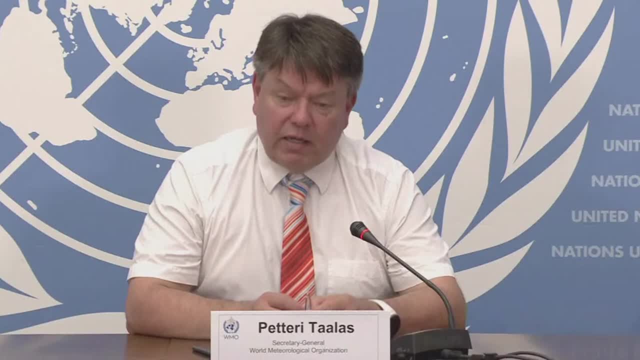 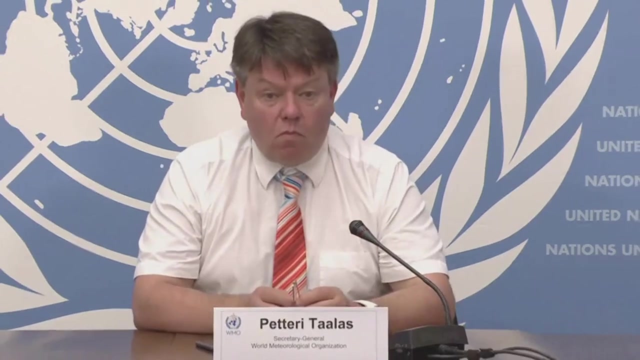 So they are thinking whether we should start taxing coal and coal fired production of goods. So this is also global trade. Yes, This is also a global issue and it's also a global carbon taxing issue. Gogi from Soleil de Dakar. 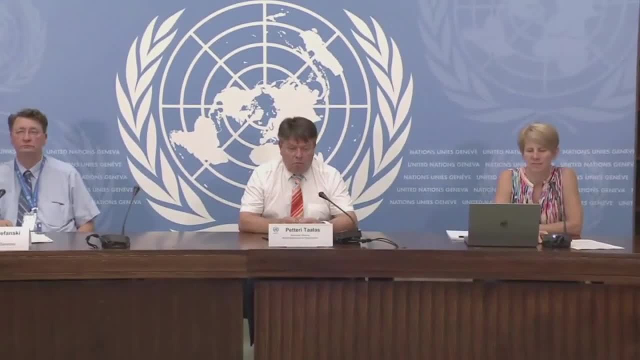 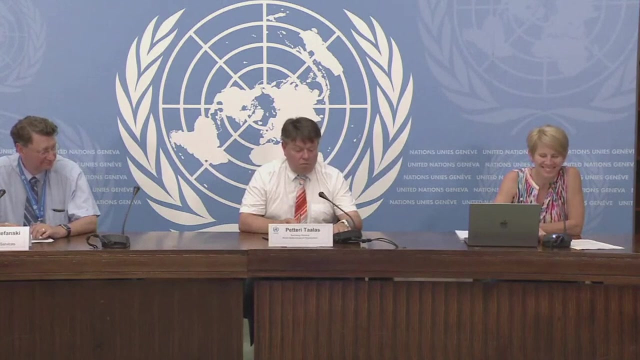 Bonjour. Merci beaucoup pour la pour d'accord My question. I think I'm going to ask it in English. Do you understand French or not? I can translate if you want. Okay, If it's not too long, Okay. 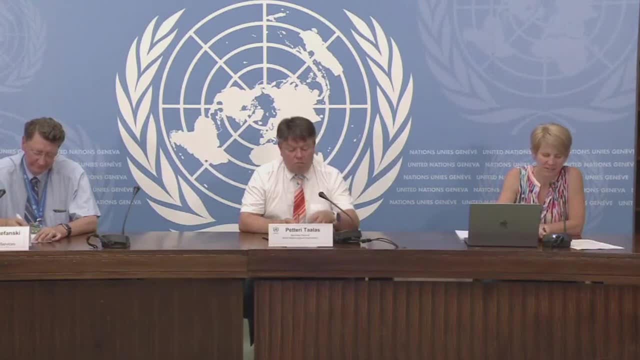 Secretary General, thank you for being with us today. My question is simple: Do we have the same heat tendency in Africa like as we have right now in Europe? And the second question: I see you are very nice with a nice shirt and a tie. 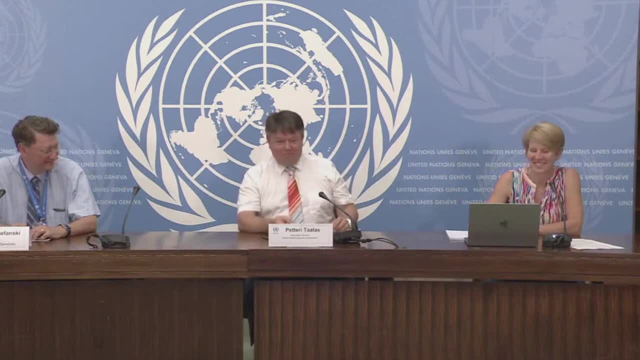 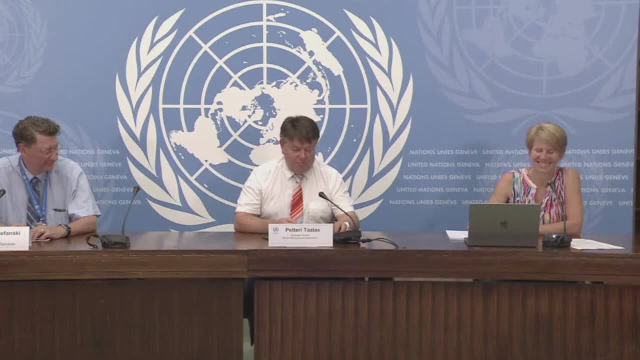 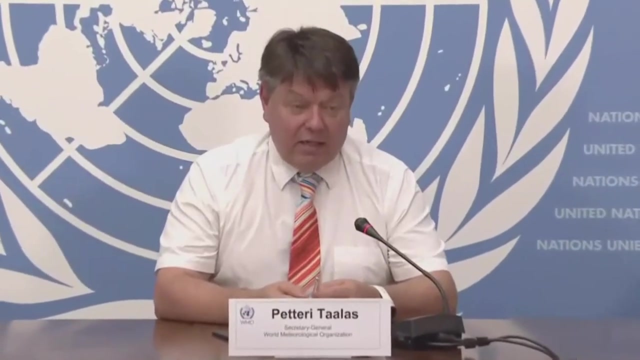 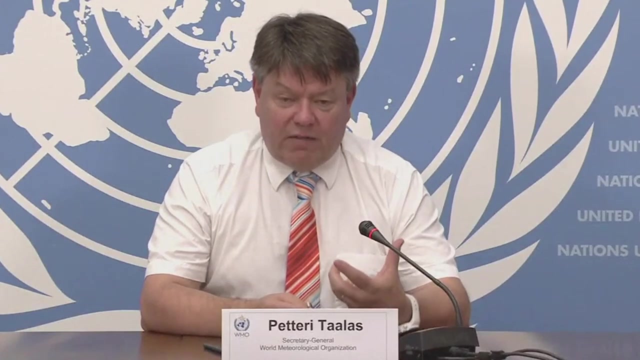 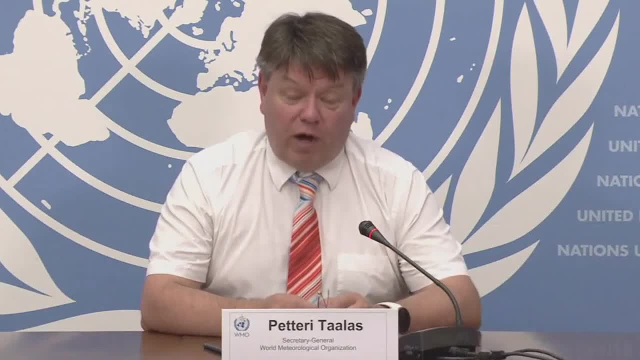 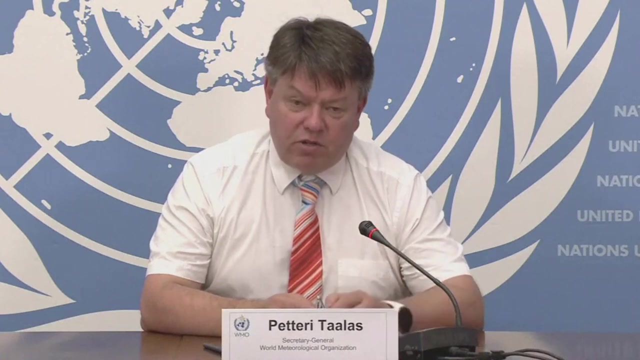 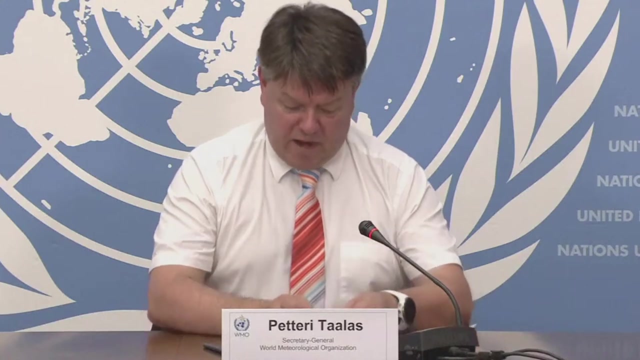 observed an increase of heat waves worldwide, And that's also covering African countries, and in African countries, the heat waves means also negative impact on agriculture, because when we have higher temperatures, we have also more evaporation, and that's bad news when it comes to yield. 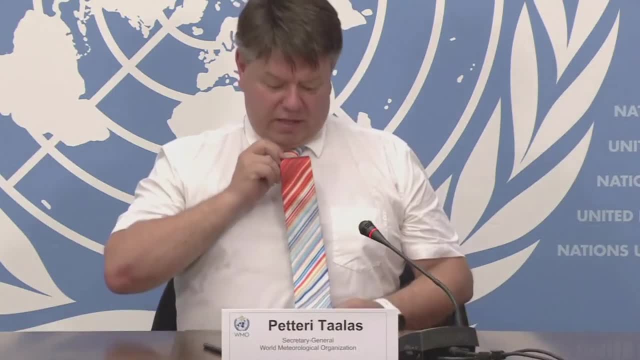 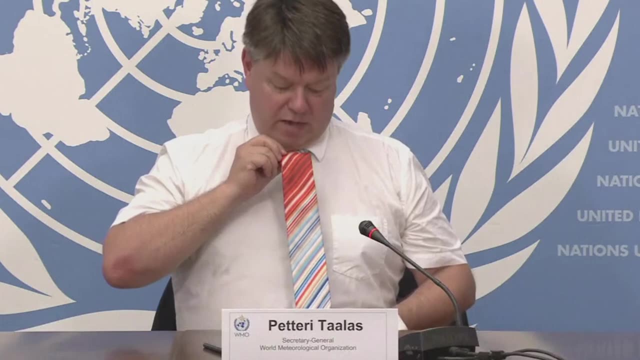 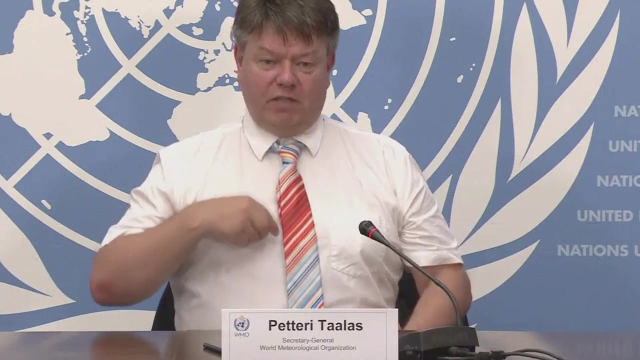 And I'm happy to wear these kind of ties at these kind of events- which is demonstrating what we have seen happening in the climate for the past 150 years. You can see that in the past we had much more blue color and more recently we have seen more red color. 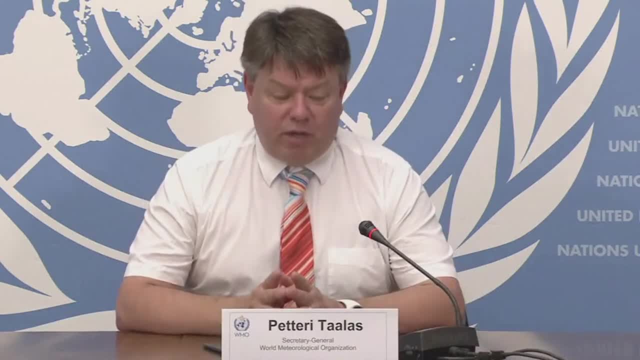 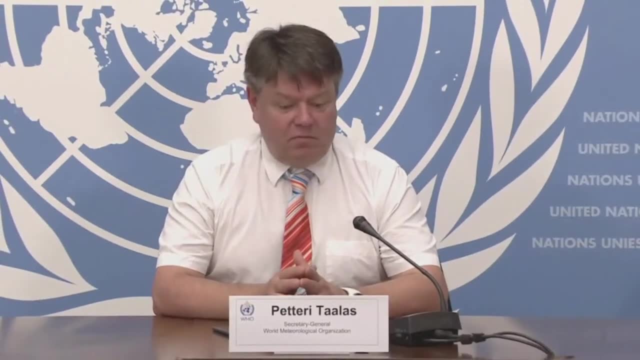 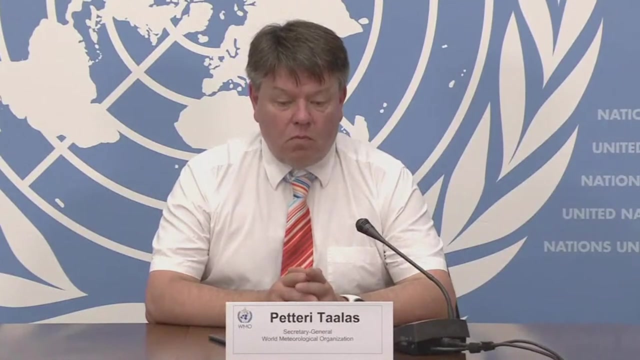 which indicates that the heat waves have become more frequent. Thank you, Now we have Christiane from German Press Agency. Thank you very much And Merci, Gorky. I was going to go into the same direction about your dress code. I salute you for having short sleeves and no jacket. 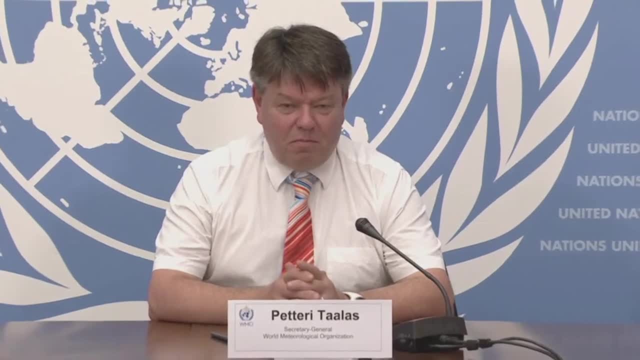 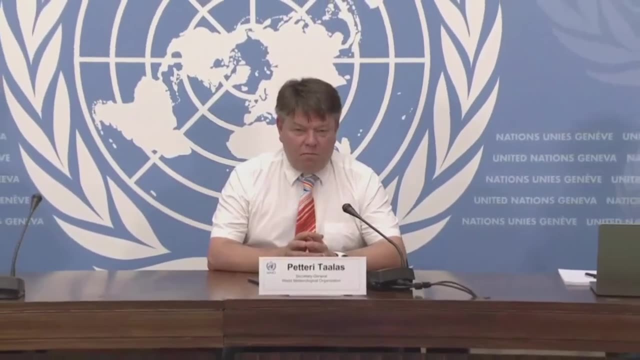 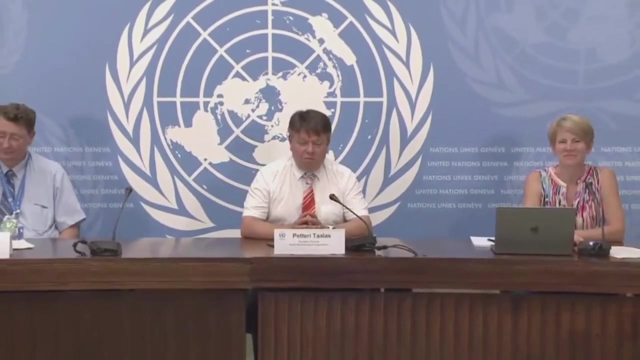 I lived in Singapore for a while, where this is the dress code for government ministers, because it's a hot country. I wonder whether you have a message for politicians in Europe and their dress code, because they seem to, and not only politicians, but many guys in Europe. 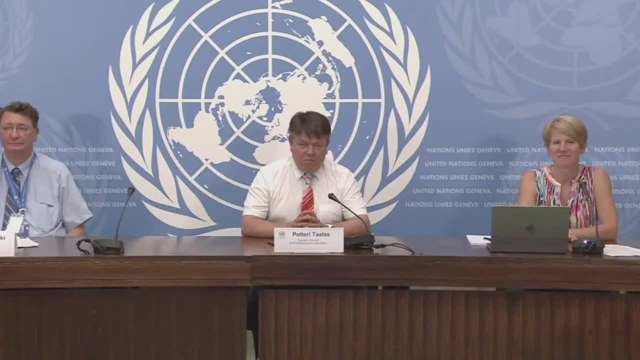 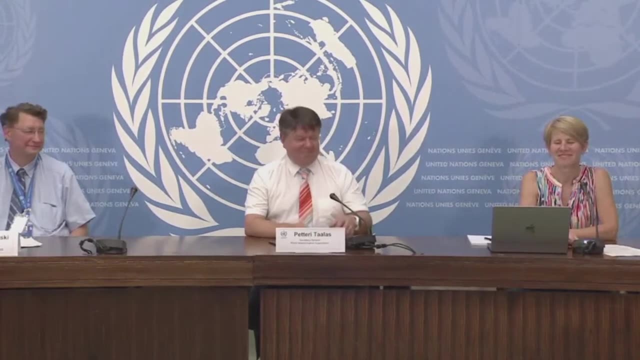 seem to have the same message. They seem to think that even at this heat, it's necessary to wear a tie and a jacket on top of the shirt. Maybe you have some advice for these people, And that might also be a message, you know, if you see your politicians in short sleeves. 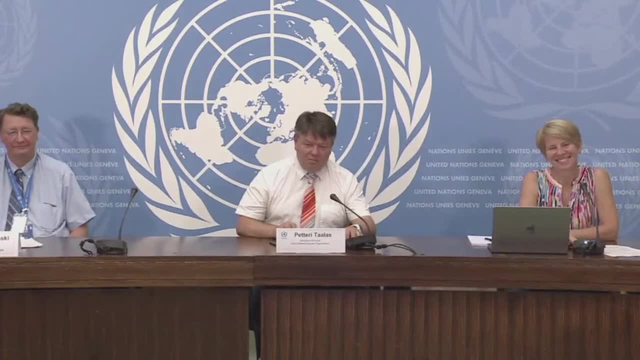 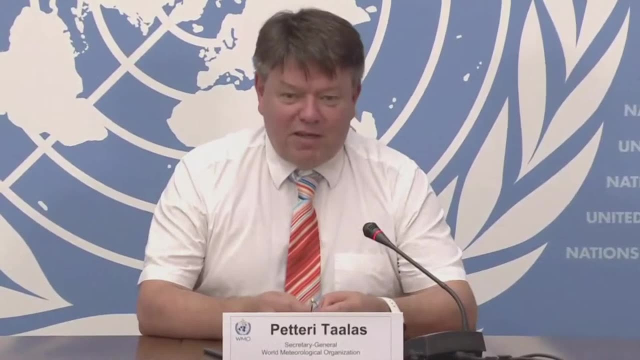 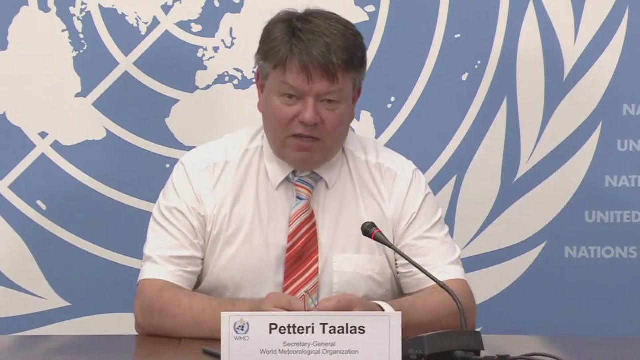 that might also be a message to people about climate change. Thank you, Thank you. That's a question a little bit out of my core competence, but this press code that we are having today it's coming from the era when the room temperature indoors was much lower. 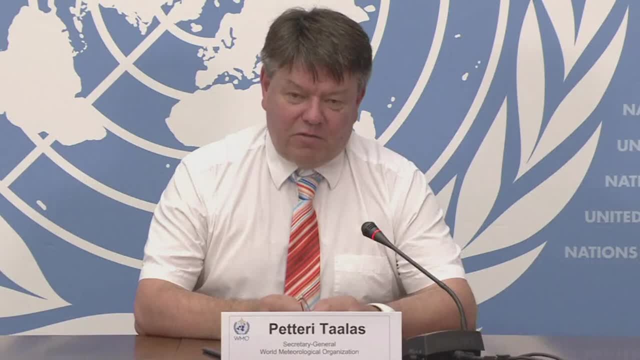 so perhaps 10 to 15 degrees, And then it was worthwhile to wear that kind of jackets. And here at the press conference room we are having perhaps 37 degrees, as is the outdoor temperature here in Geneva today, And it's more comfortable for the functioning of the brains to wear this kind of jacket. 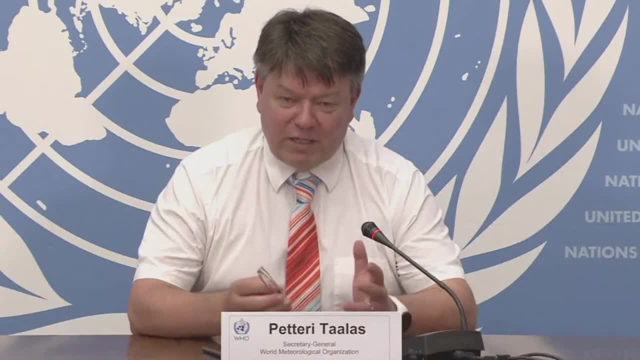 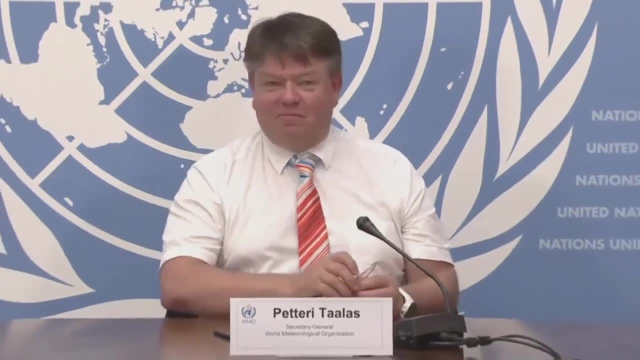 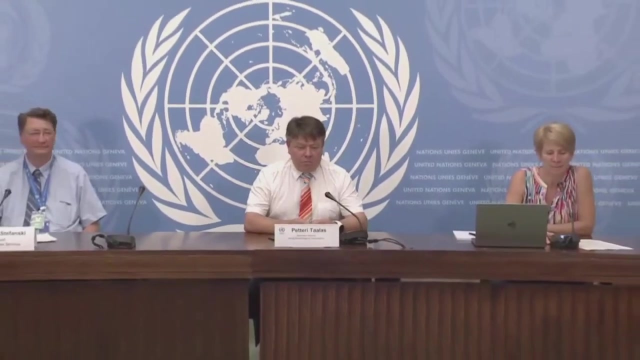 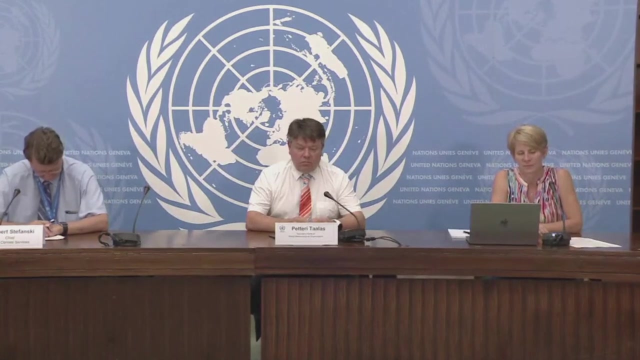 So if you are very disappointed with that, I'm sorry for that. We will take a last question for our secretary general and then he will have to leave. From Emma Farge, Good afternoon. You mentioned the glaciers. I was wondering if you could talk about the bigger impact of melting glaciers. 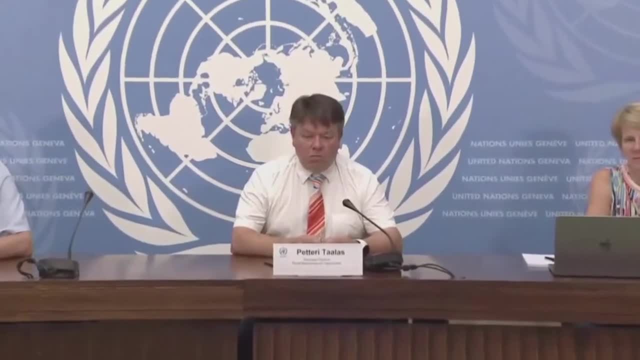 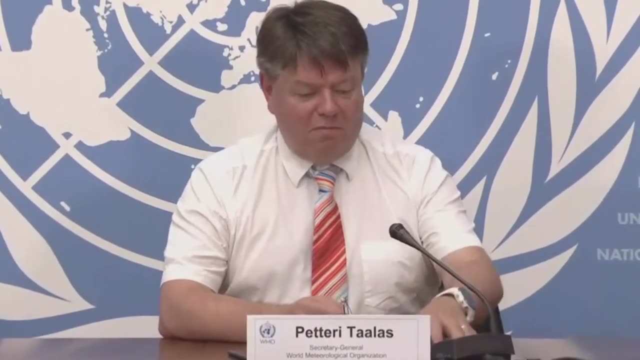 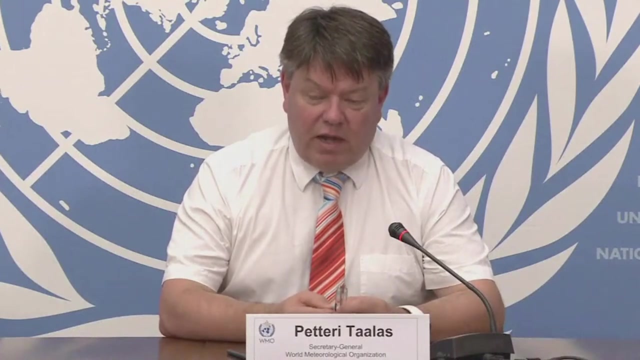 What do you expect that to be in the future? And is this the opportunity to start naming heat waves? What would you name this one? Thanks, That's a good question. So, as I said, we have already lost this glacier game. 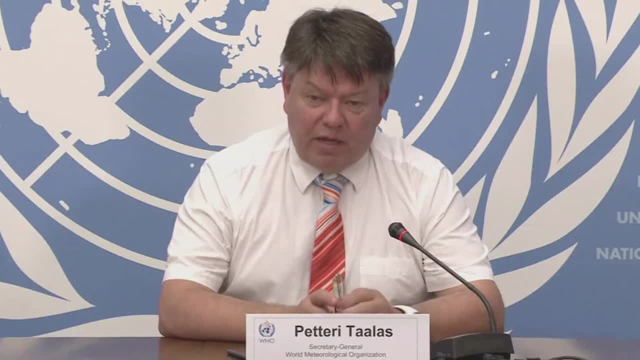 And if you look at the statistics for the coming decades, we have seen glacier melting intensifying, which means that we are having less and less water in the mountains, glaciers worldwide, And we have also started melting the biggest glaciers in the world, especially Greenland Glacier. 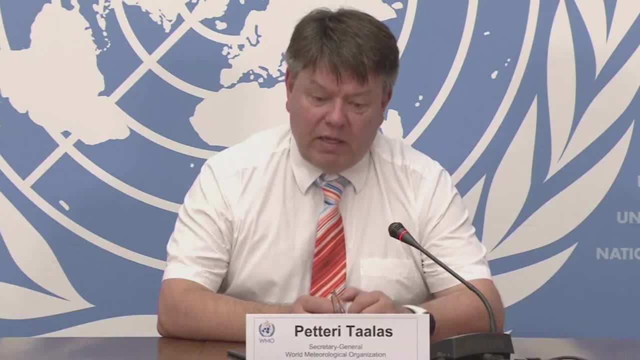 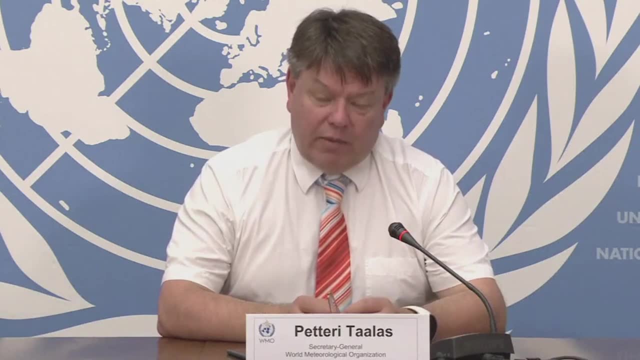 There has been a major boosting of its melting And also the Antarctic Glacier, where we have the biggest ice mass worldwide, has started melting And we are going to see both local impacts and global impacts because of that. The global impact is going to be sea level rise. 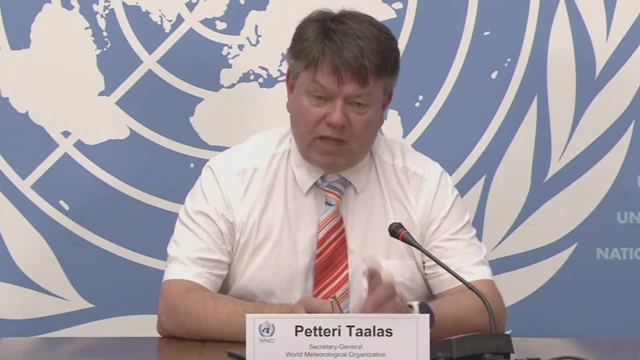 which has been already boosting. So 20 years ago sea level rise was about two millimeters per year, whereas recently we have seen 4.5 millimeters per year sea level rise, And this is very much coming from this speeding up of the melting of glaciers. 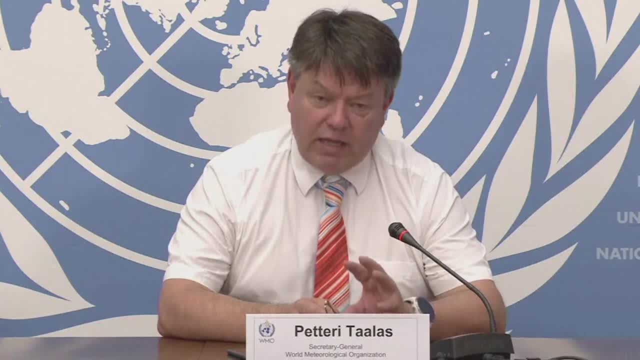 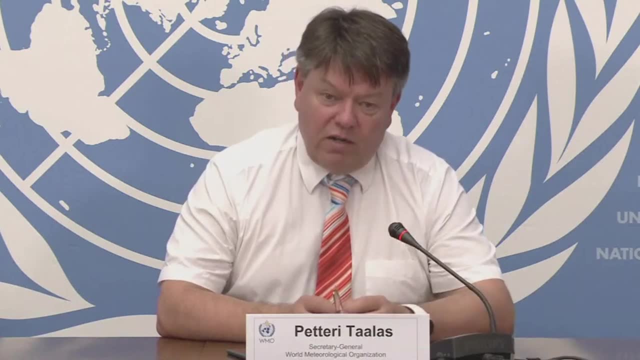 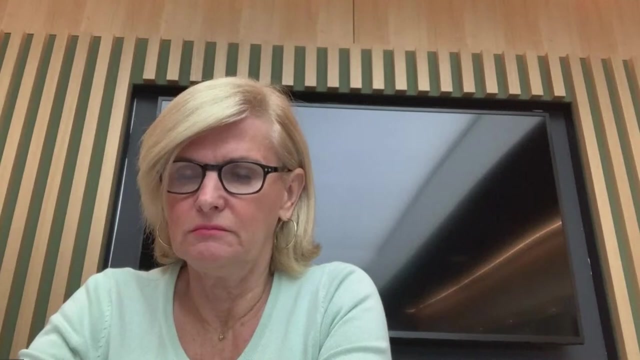 And this is having global impacts on island states, low-lying areas, big cities Which are on coast, also in London, where you are, Maria, at the moment. But besides that, we are going to see local impacts Many of the big rivers worldwide. 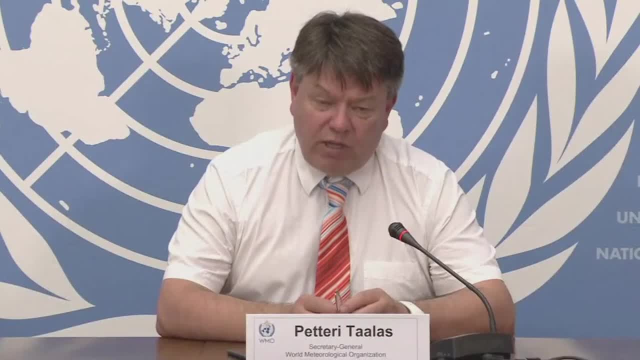 they are having their origins from melting glaciers And, because of the shrinking of the glaciers, we are getting less and less fresh water to the rivers, which has a negative impact on agriculture, on human health, on water availability and also for industries. 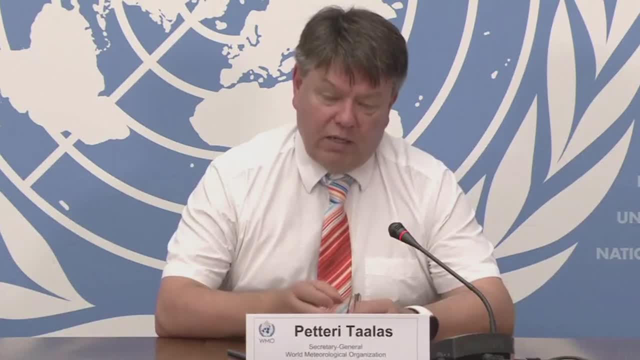 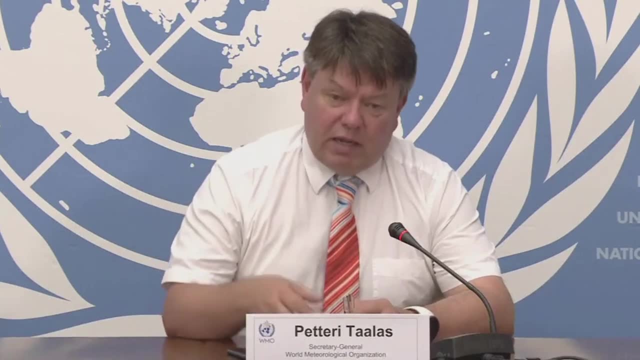 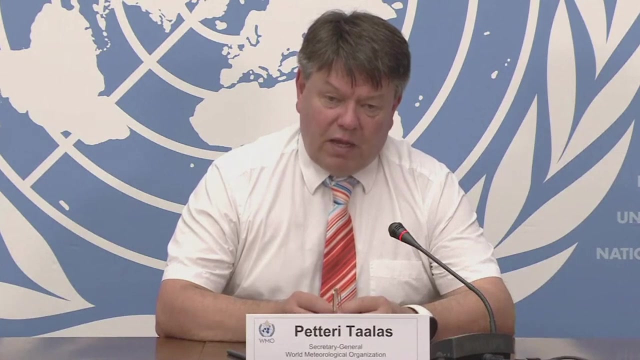 And that's happening also worldwide, And we have major glaciers in the Himalayas, here, Alps, then we have Andes and then Rocky Mountains in America, And in all of those cases that's happening And this will mean bad news for the coming decades. 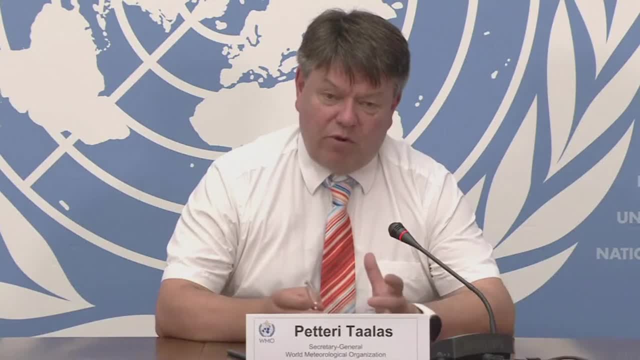 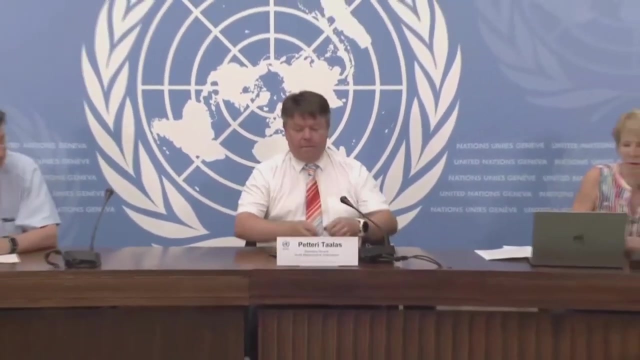 and also for the coming centuries. For example, here in Europe we expect that the melting glaciers will mostly disappear by the end of this century. Thank you very much. I think you need to go. Sorry about that And, Bob, maybe you can answer to the question. 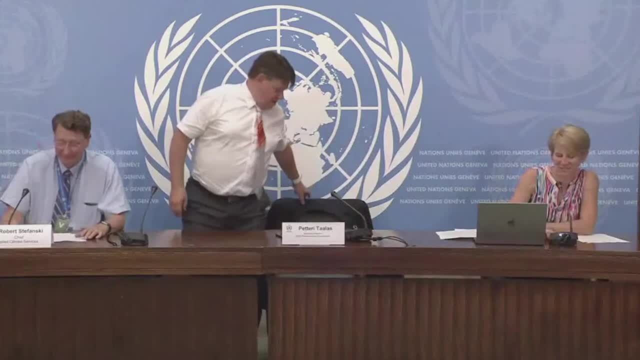 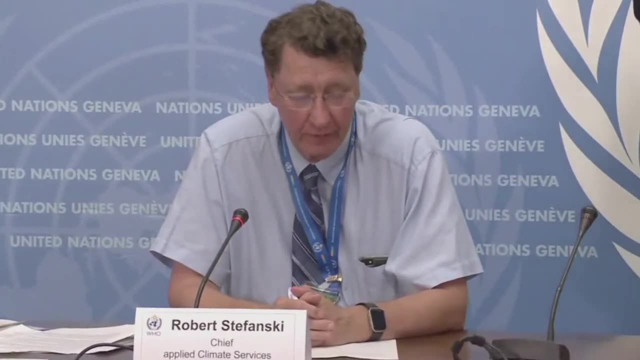 on naming heat waves, Thank you. Thank you for the question. So we have a good collaboration with WMO, WHO and a number of the national weather services around the world. We have something called the Global Heat Health Information Network and also a joint study group looking at this issue. 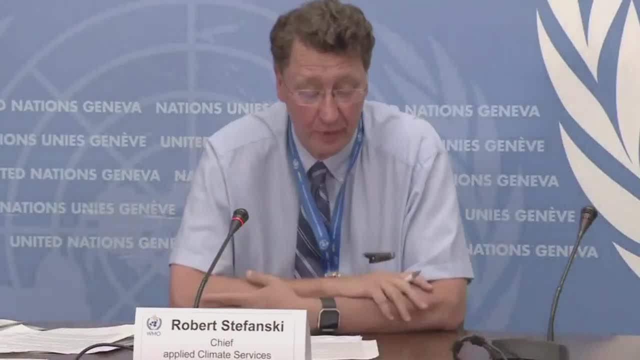 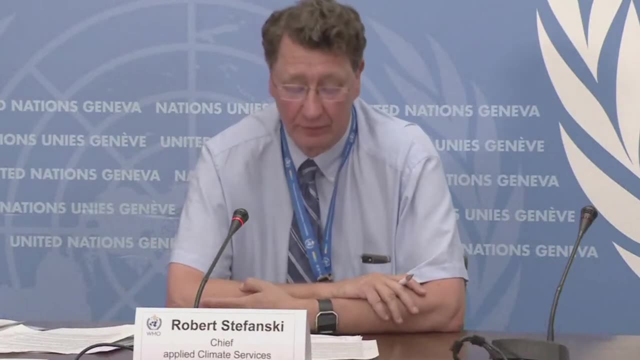 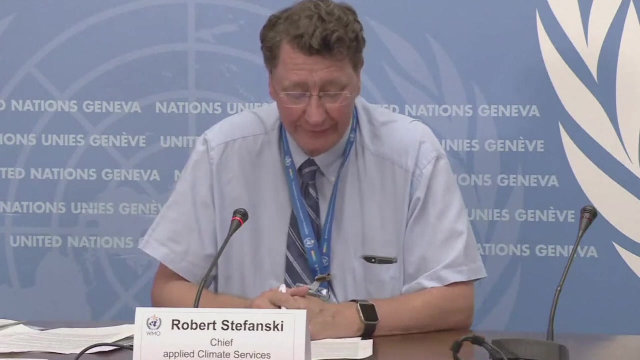 And so currently there's no plans, at least for WMO or our partners, to name heat waves. Heat waves are not like tropical storms. I mean, these tropical cyclones or storms are very specific and very discreet, So there's caution. 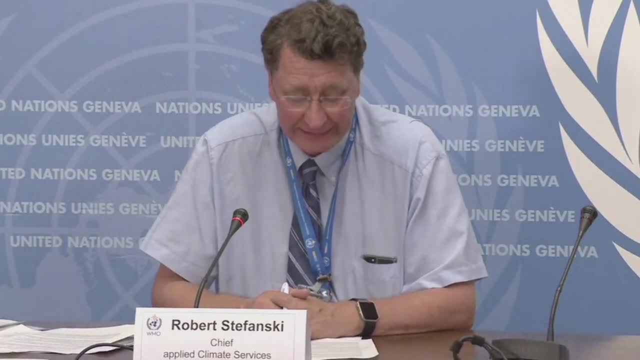 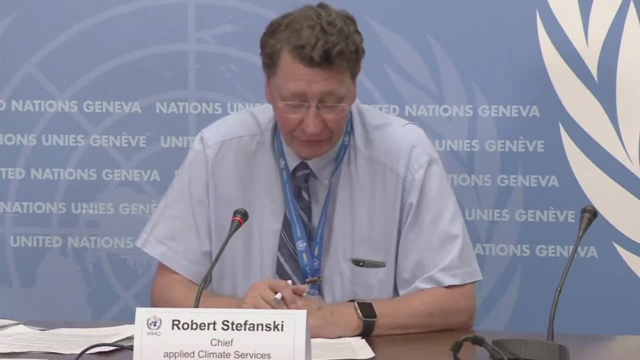 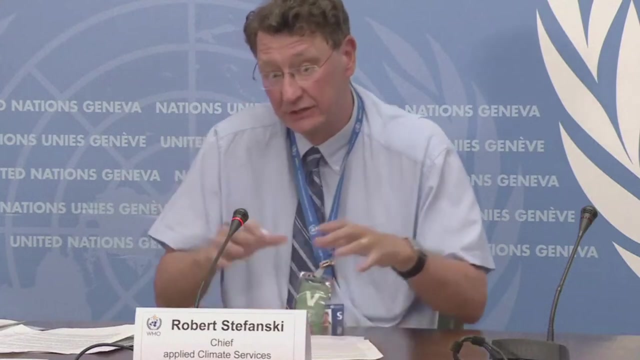 We advise caution on trying to use this for heat waves Specifically, you know, naming heat waves causes additional challenges. The named events may not take place, They may turn out to be less severe and may not occur in different localities. So again, the definition also of a heat wave may vary. So trying to do that is quite difficult. I know a number of the weather services, especially Medio France, tries to characterize the major heat waves by year And thus far in the climate community we've been able to identify the major events across the world. 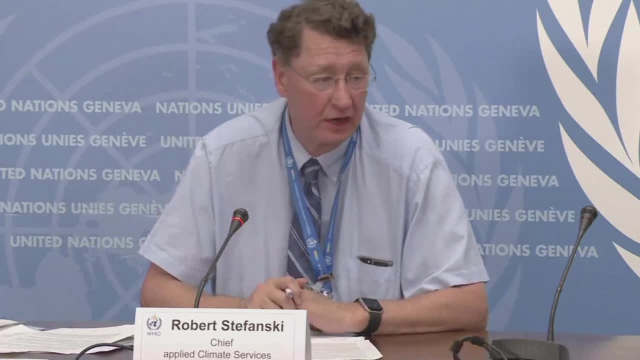 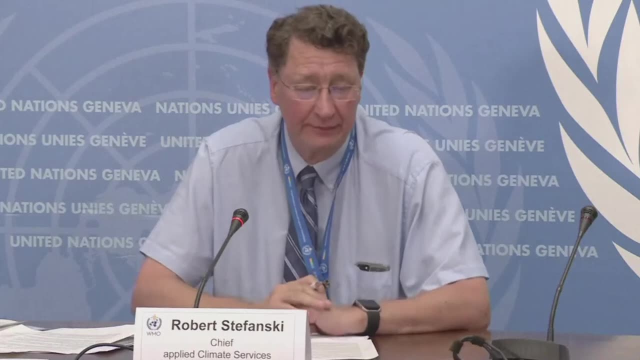 And, as this current event shows, you know, nations, the weather services and national health authorities are doing a very good job with health warnings on heat waves and making people go to shelters and the measures that Maria talked about earlier. So currently there's no plans. 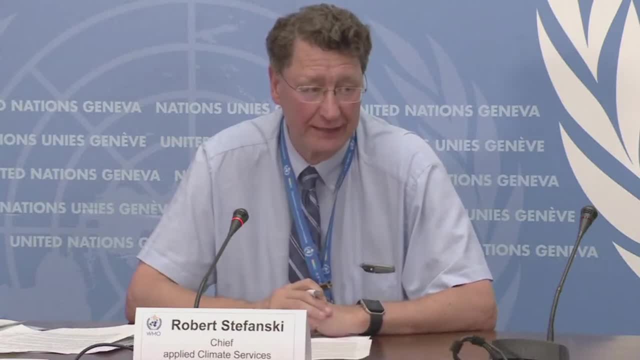 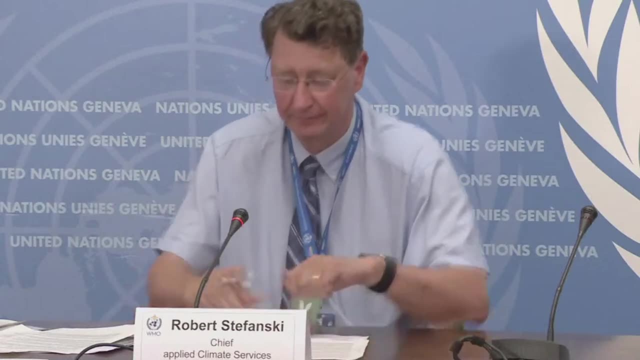 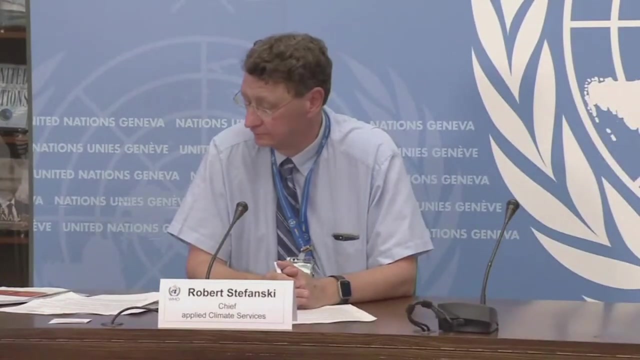 because it's a very difficult issue and we don't see a way to make the public messaging very clear on naming heat waves. I hope that answers your question. Thank you. Now we can open the floor to any more scientific technical question. Yes, please go ahead, Christophe. 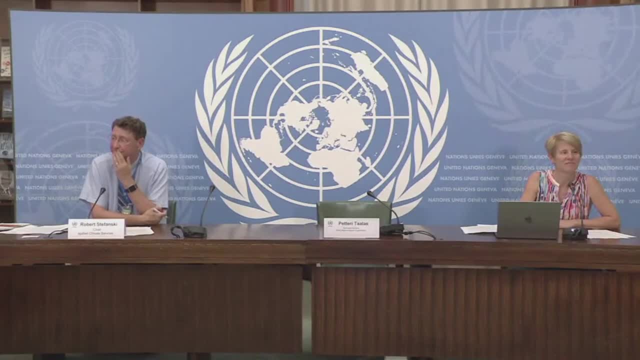 Thank you. The question is for Dr Neera. I was just wondering if you have an idea or an estimation of the number of victims that the heat wave like the one we're experiencing right now can make in terms of heat but also, as you said, pollution. 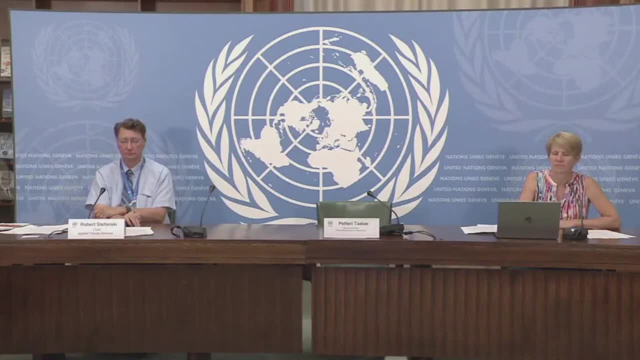 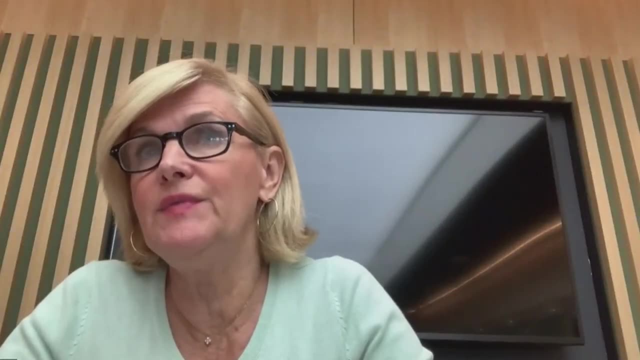 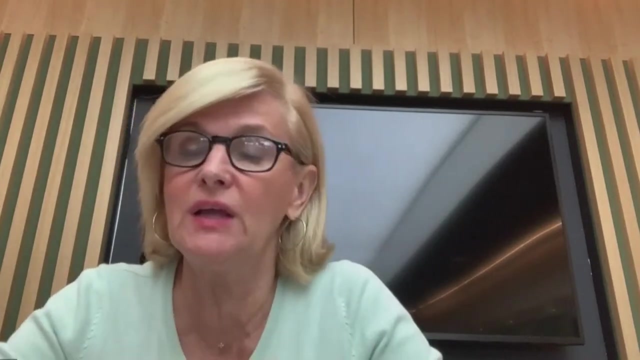 And if you maybe could elaborate a little bit, Thank you, Thank you very much. We are having now very daily notifications of the number of deaths country by country, but we don't have a final figure, But if we know that in 2003,. 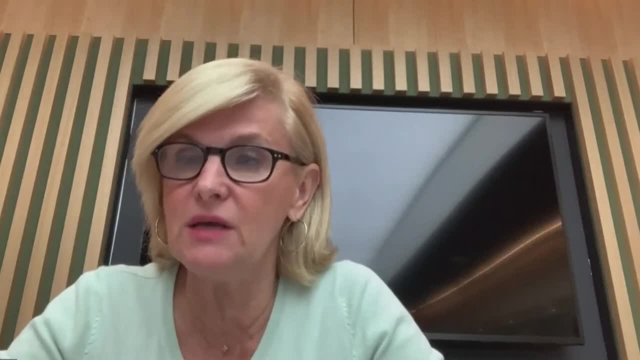 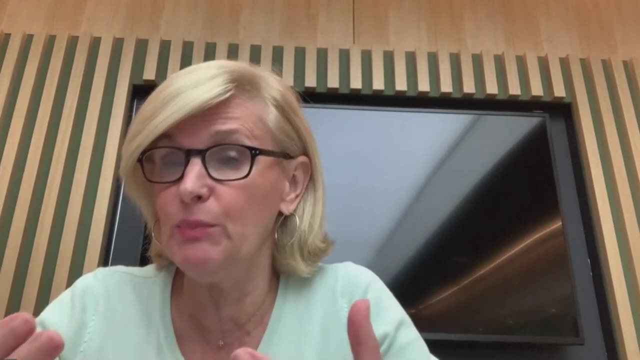 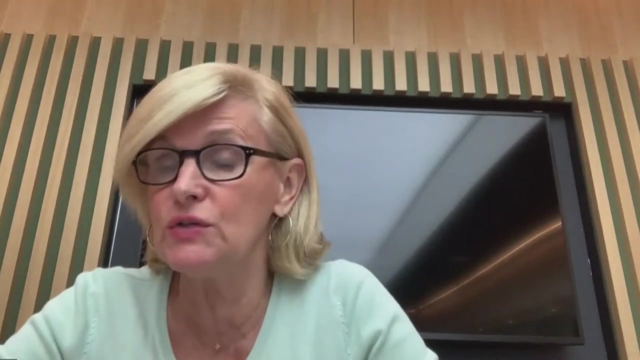 as I mentioned, the figure was very dramatic: 70,000 deaths. Even if now, maybe in terms of early warning and alerts, we are better prepared and the cities are much more on the proactive search for those cases and releasing awareness, raising messages for the population. 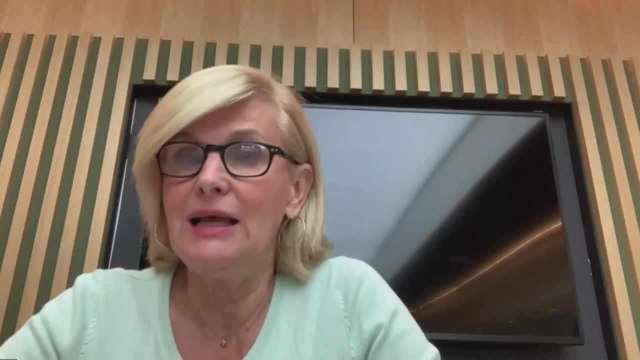 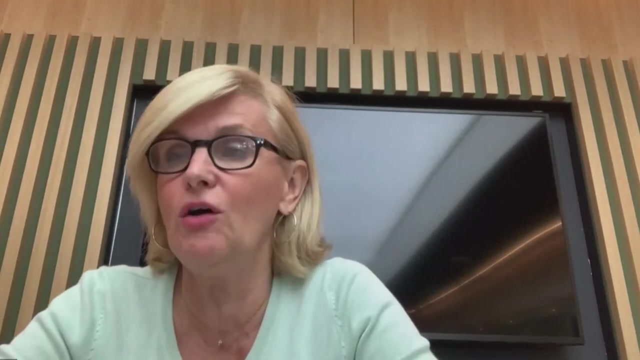 I'm sure that will be a big figure, But again I think we need to use this very strong signal that again we are receiving for accelerating our action to look at the causes of this global warming and these heat waves And although we need to adapt, 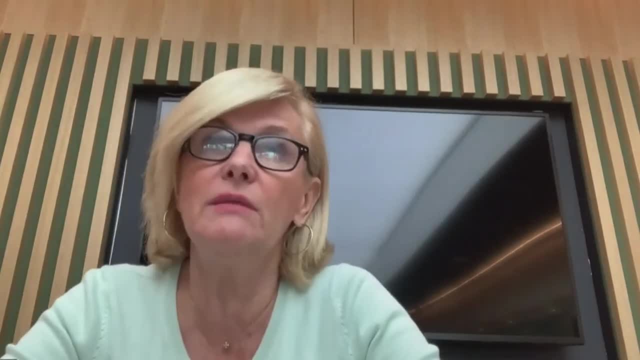 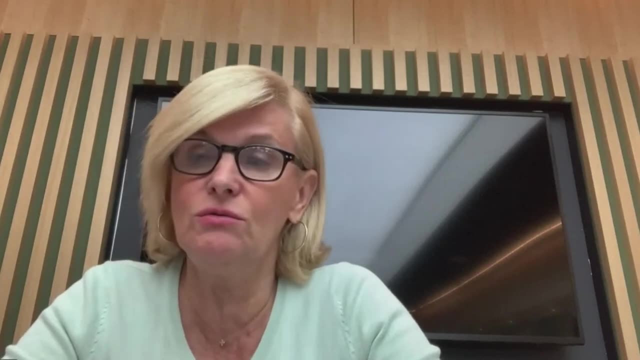 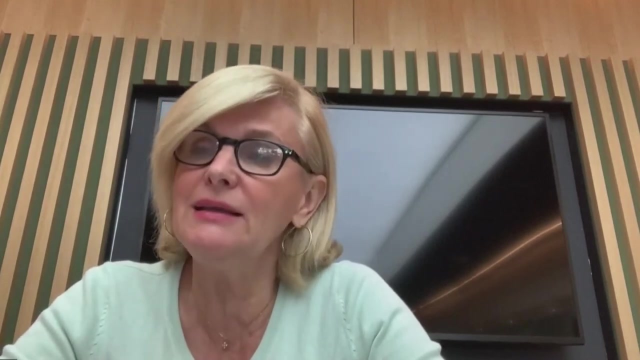 and prepare better our cities, because cities is where probably we will be having more problems and they need to take at the urban level many actions to adapt ourselves, and that the cities are not prepared at the moment. We again, the call is for responding. 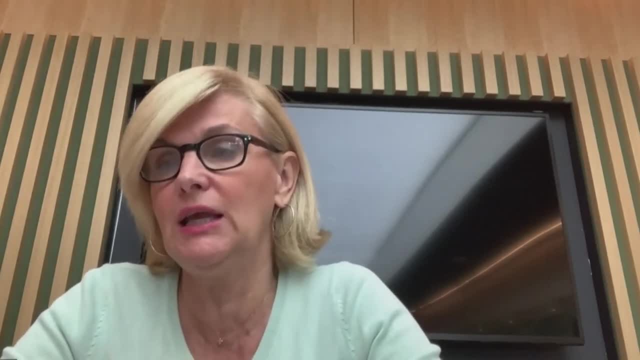 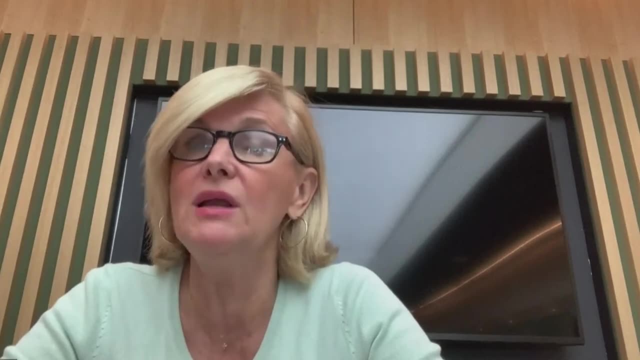 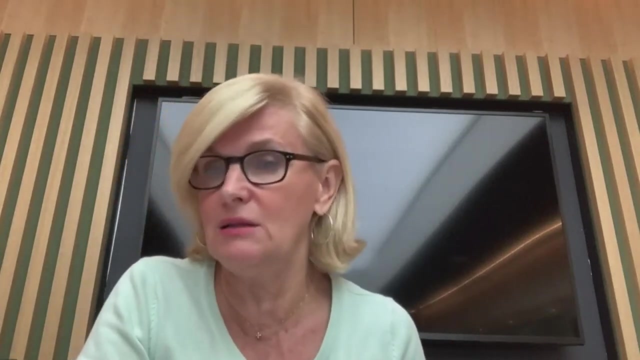 to the very acute situation, but looking again on a very serious and ambitious way, tackling the causes of this global warming. Climate change is affecting our health from many, many ways, not only by the heat waves, which are a direct consequence in the number of diseases. 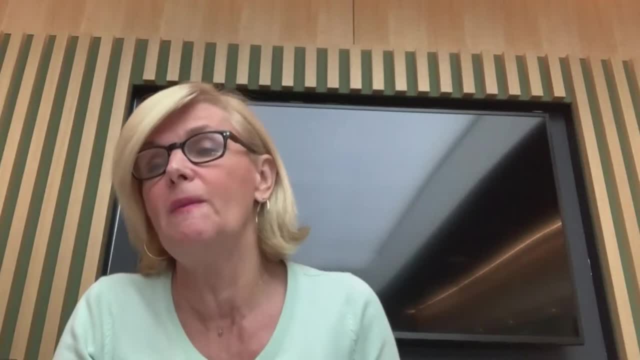 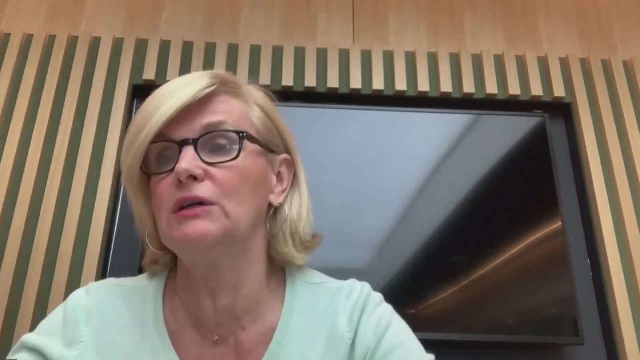 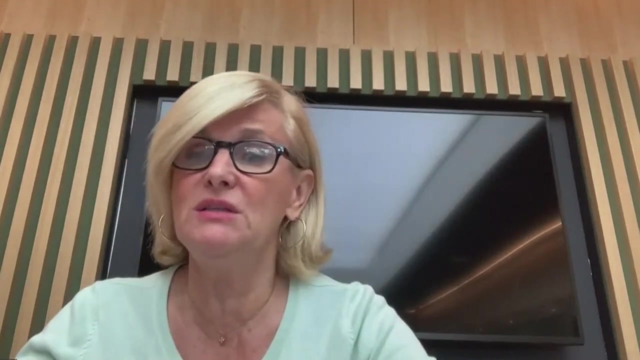 and conditions that is causing, but as well, because it will be touching the pillars of our health: the access to food- We will not have a good agricultural production. access to water- There will be water scarcity, for sure. There will be more diseases transmitted by vectors. 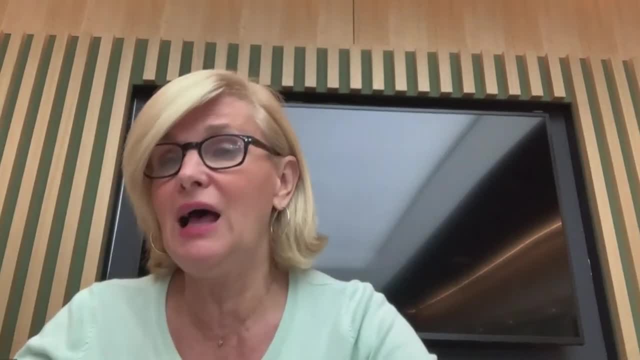 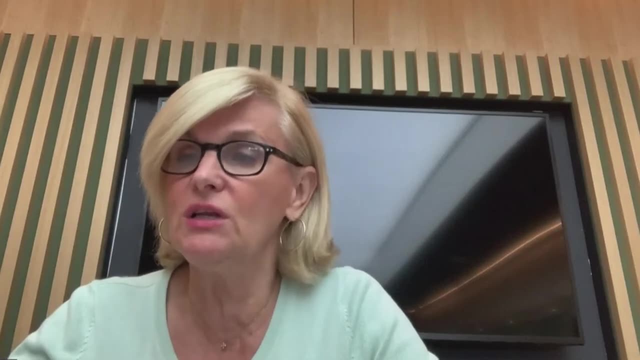 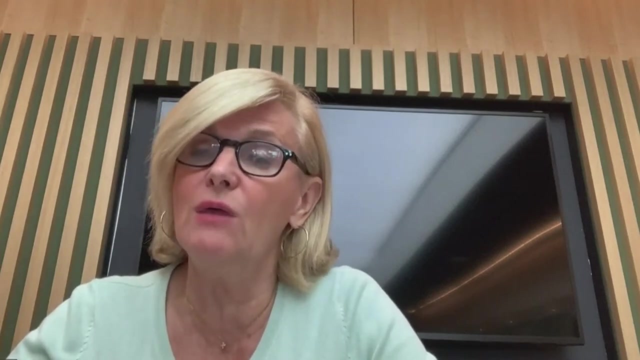 because of the weather conditions, There will be a crowded situation in our cities and heat stress And there will be definitely migration and social inequities and problem with our quality of the air we breathe, which is already very much affected In terms of air pollution. 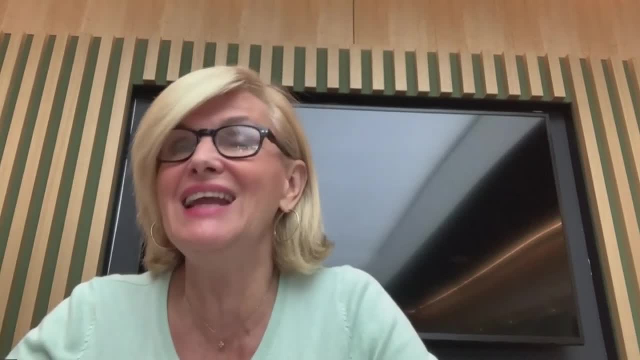 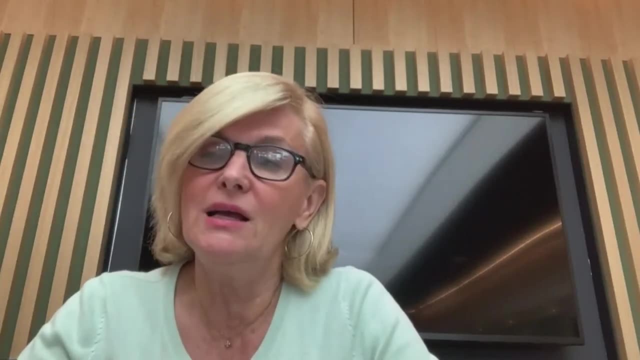 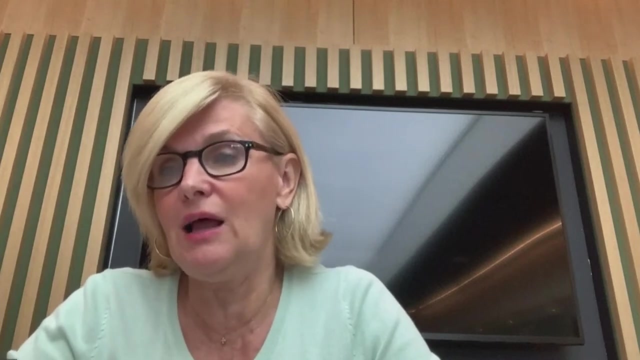 as you know, at the moment, according with our standards, 99% of the global population is breathing air that is not respecting the proposed standards by WHO, by air quality guidelines, And therefore we would like to see, as well, less dependence on fossil fuels combustion. 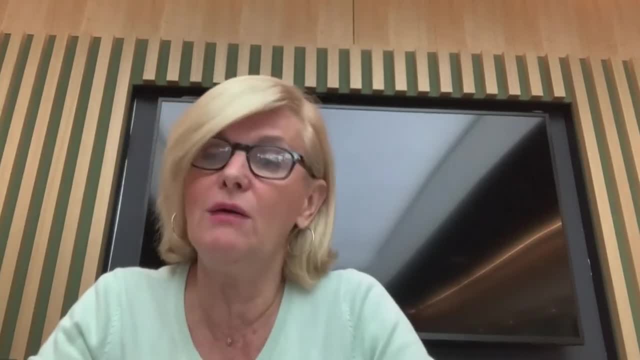 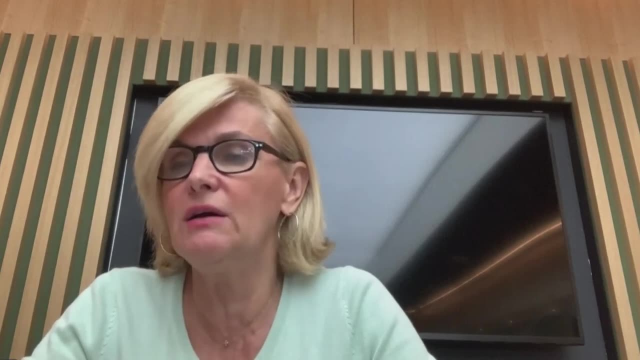 because this is putting at risk our planet, our climate change, but at the same time causing major pollution and therefore affecting on a very important way our health. Thank you, Emma, And please mention to whom you direct your question, If it's for Maria or for Bob. 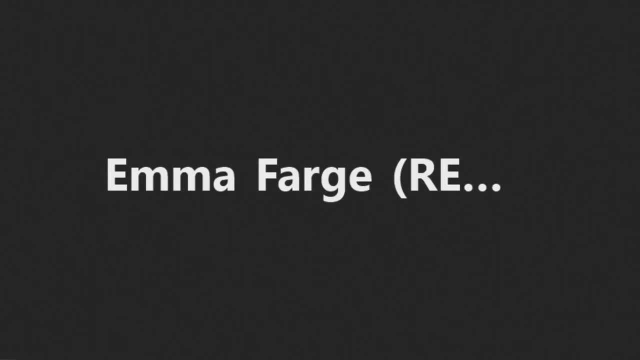 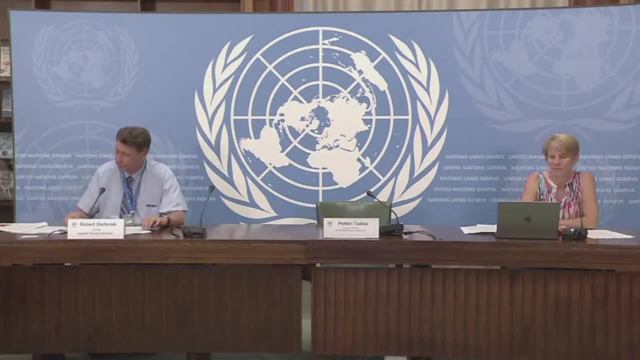 It's sort of for both. I was hoping they could elaborate a bit more on the health challenges with the pollution, So that one would be for Maria but maybe for Bob. Do you have any data on the deterioration of the air quality due to this heat wave? 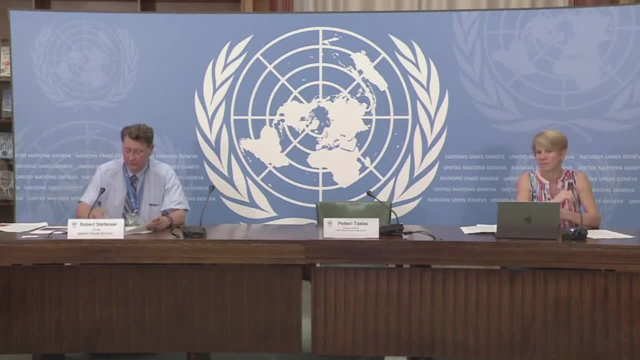 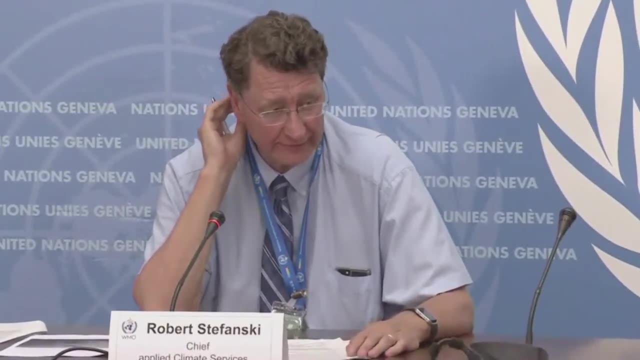 Or could you elaborate a little bit more on the trend that you've seen? Thanks, We don't have any data at the moment, But, as we do know again, if anybody flies or goes up in elevation with any mountains in Europe, you can see the less. 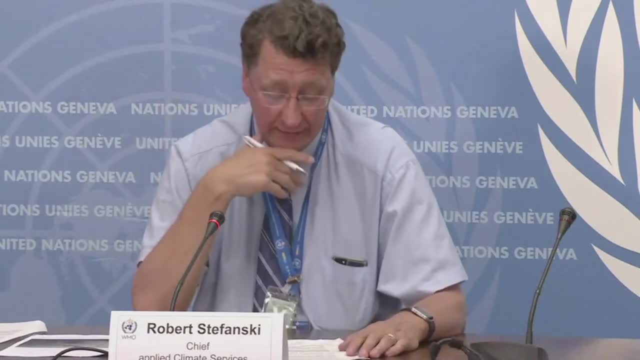 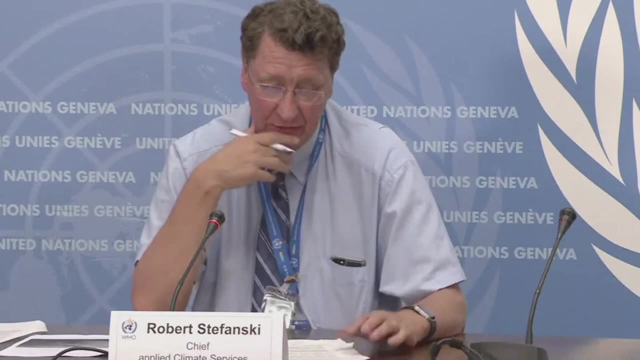 you know a lot of you know less visibility in the air, So I don't have any data. Again, this is a cumulative effect And Maria knows can talk more about that. But again, under these events the air becomes very stagnant. 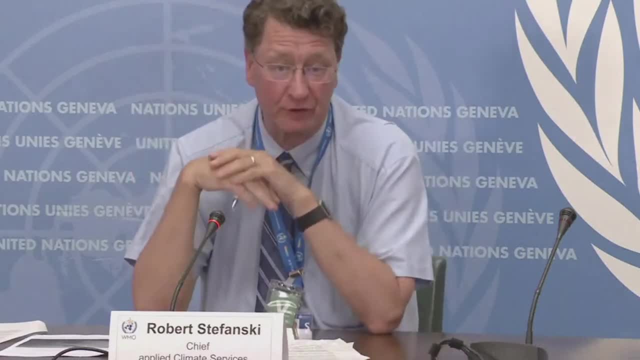 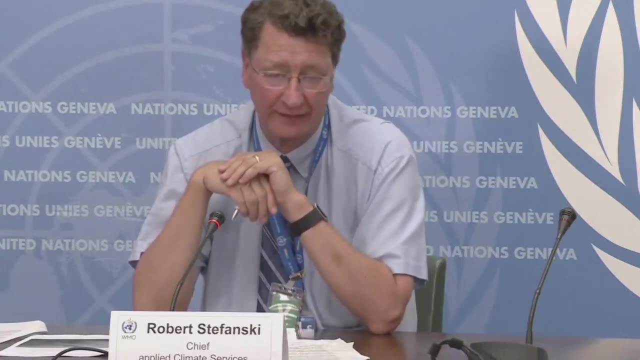 And actually the air is coming down to the ground and that traps all these pollutants and also makes for the heat wave. So I'll let I'll let Maria maybe answer more questions on that, But we don't have any specific data right now. 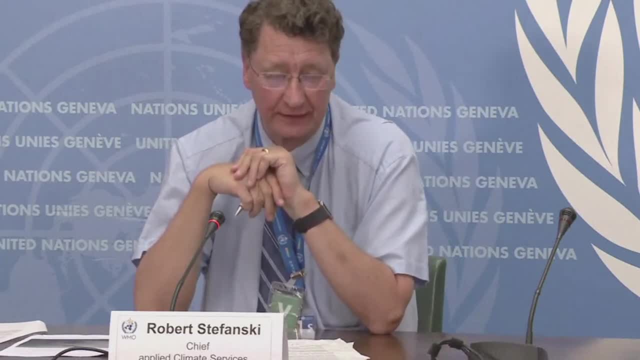 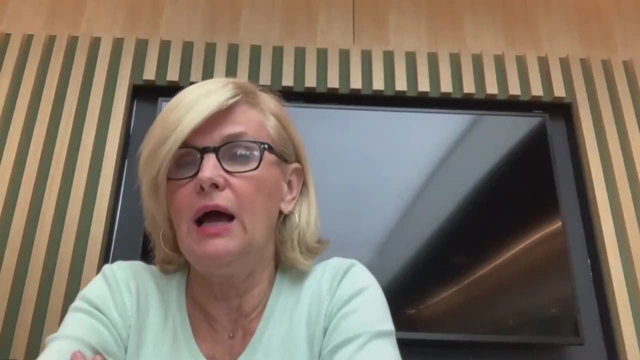 Again, as you can anticipate, it's a current event, So we're trying to get some of the data and the air quality measures as we speak. Thank you. Yeah, thank you, Robert, I agree. I mean we have data about the levels of air quality. 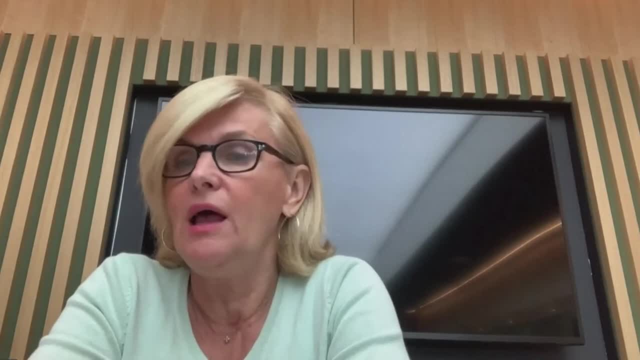 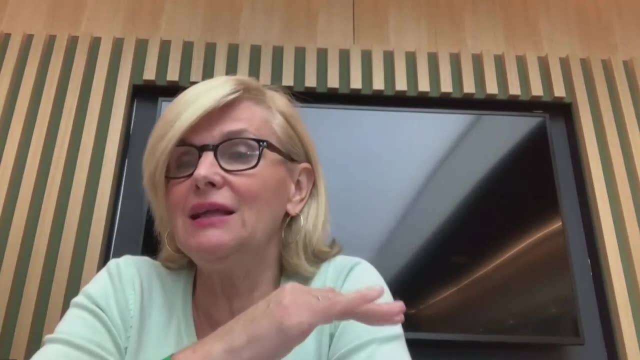 in most of the cities around the world. There is a very good monitoring system in many, many cities, and particularly in Europe, So we can know the levels of air pollution every day. But now how this interacts with the fact that the heat wave. 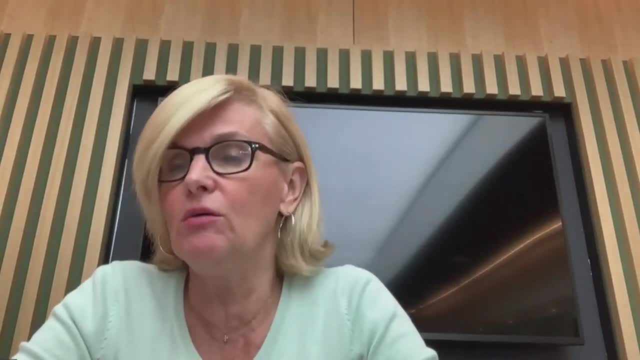 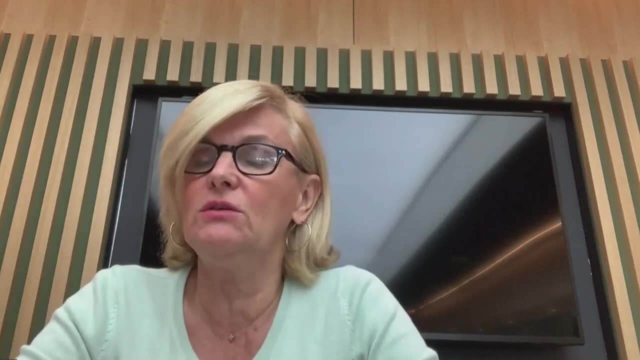 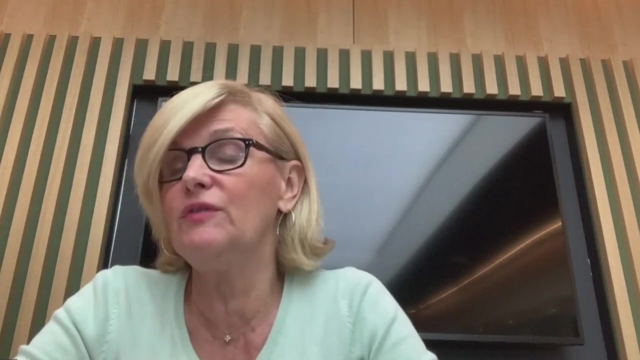 and data about that will become cumulative and we will see, But for sure, the people with chronic respiratory conditions. this heat wave will aggravate and exacerbate this situation And, for cities that are very polluted, the fact that, in addition to the pollution, there will be this heat wave. the heat and high temperatures will certainly make the respiratory conditions- the acute ones, more serious In the medium and long term. this is what we are very much concerned For: how long an individual is exposed to bad levels of. 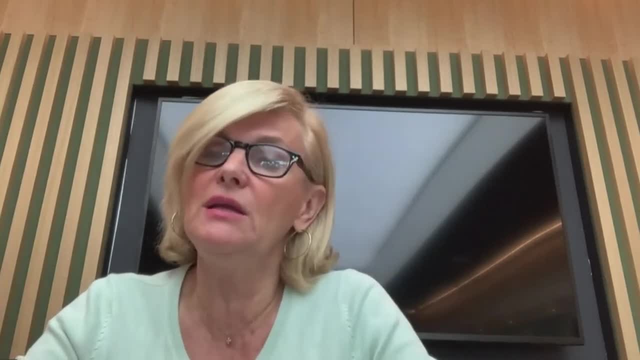 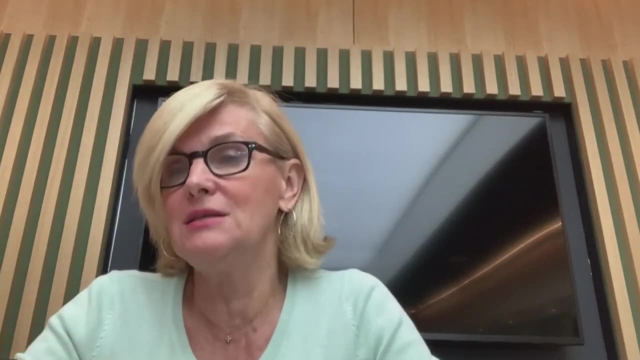 I mean high levels of air pollution And then we can estimate what it represents for the health of the people. But we see an increase on the people demanding the health system. I mean an important increase of people seeking for assistance at the healthcare facilities. 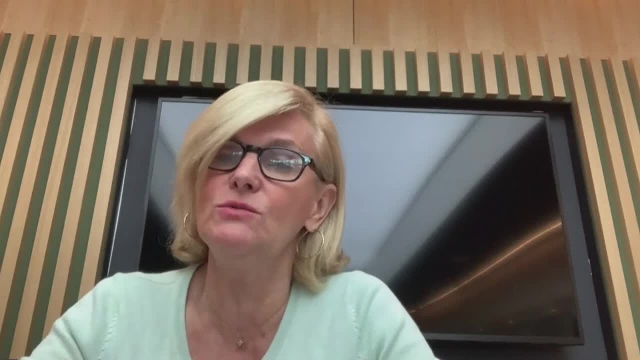 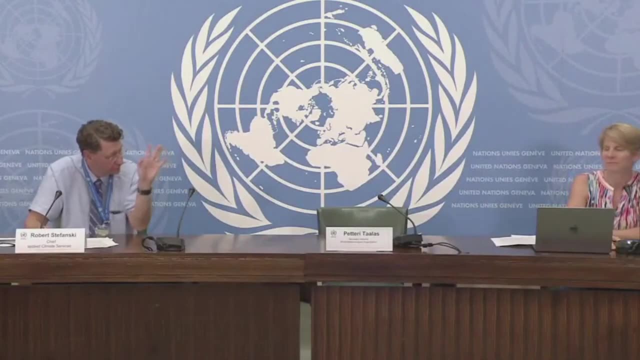 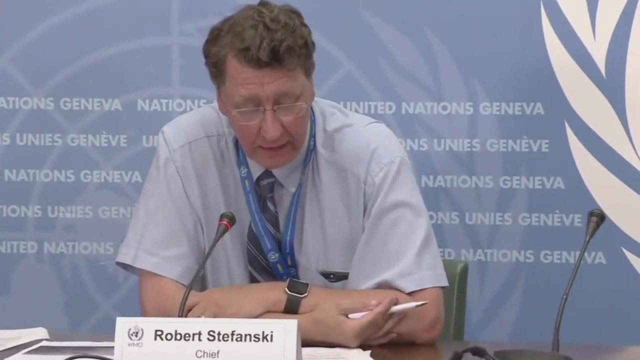 and the health sector is much more demanded these days, when there are peaks of air pollution and heat waves. Just to follow up, I didn't have any specific data for the current event, but Maria is quite right. In fact, if you look at the Medioswiss app, 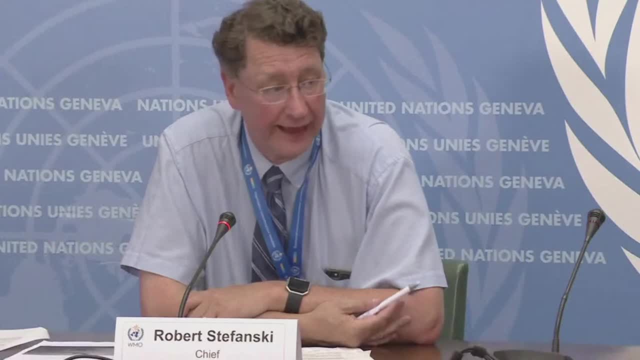 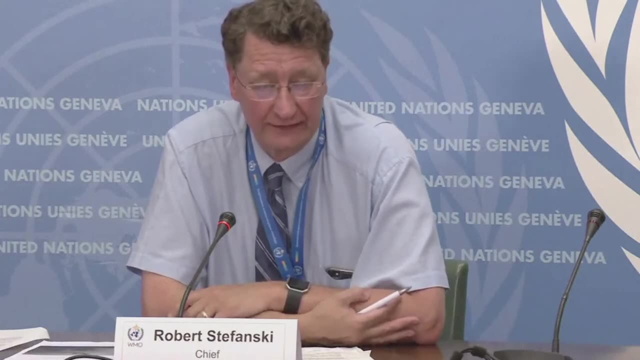 there are links to air quality apps and other websites, So it is very much connected. you know weather, climate and health across many of these sectors. So I just didn't have actual numbers for today or this week, But, as Maria said, 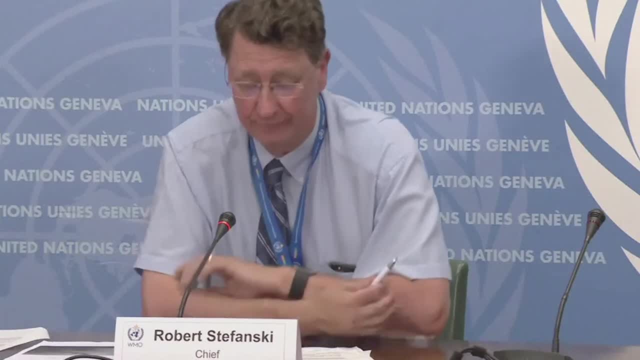 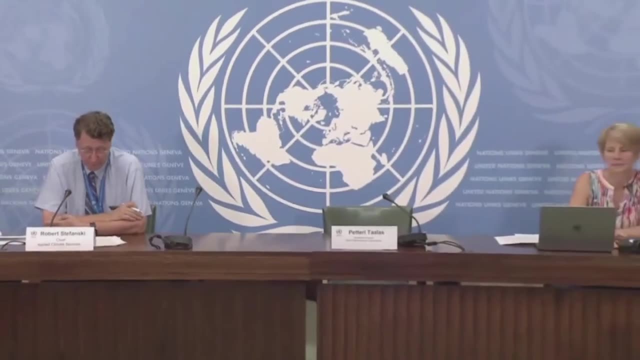 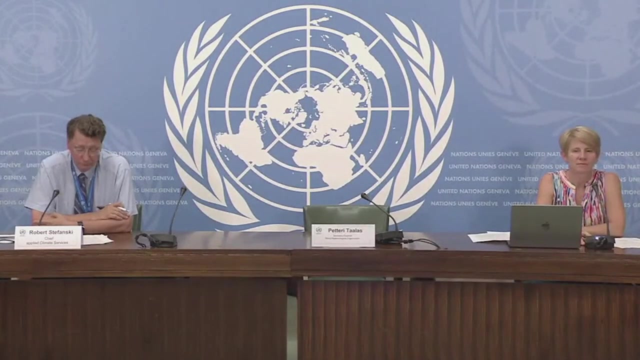 there's a good network across the world on this. Thank you, One more question from Gabriella Sotomayor. Yes, thank you for taking my question Again for Maria, Going back to the dress code now that you are there in London. 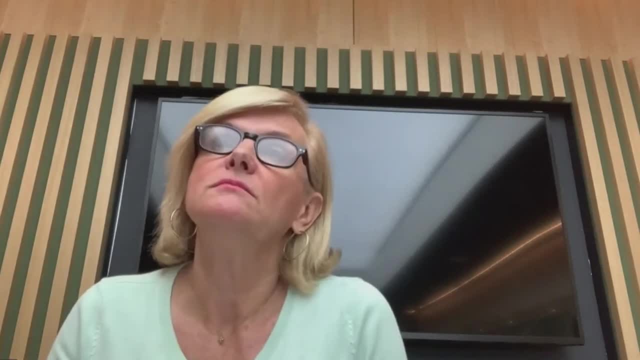 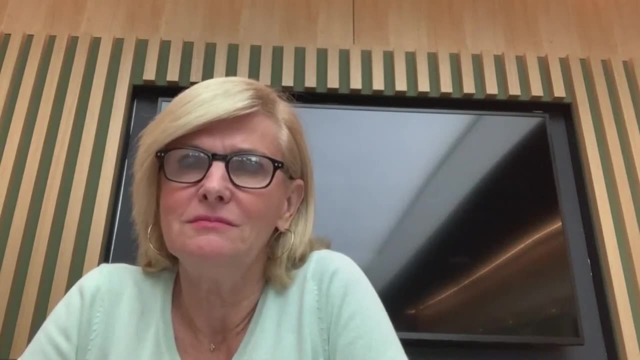 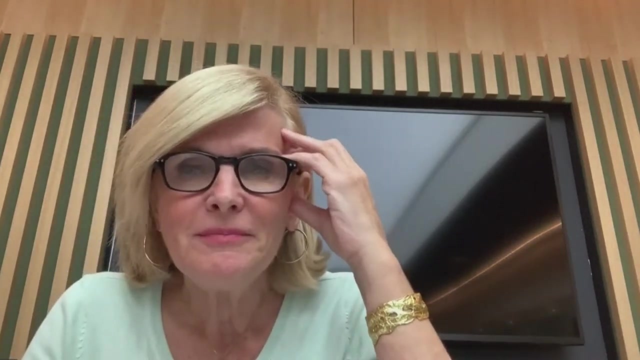 I think the Queens guards are wearing these iconic uniforms in the sunshine, So isn't it dangerous for their health? What can you say about this? Sorry, sorry, Gabriella. I couldn't hear the second part. They are wearing what? I think they are wearing these iconic uniforms. 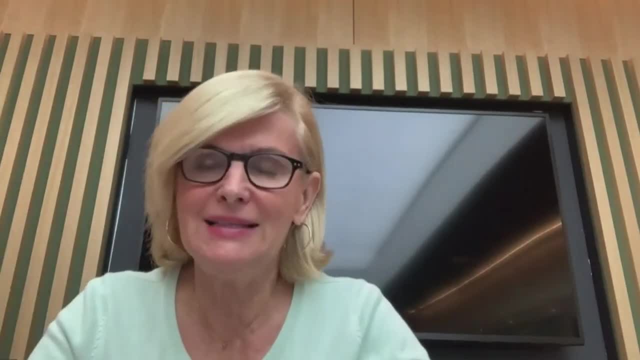 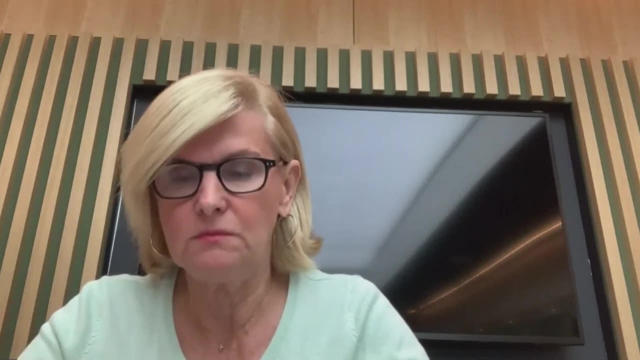 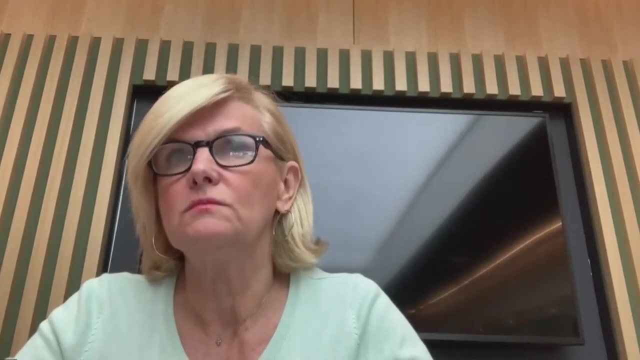 the Queens guards, Oh sorry. So I mean they are wearing these uniforms, but it's an important issue because they are there in the heat wave with these uniforms. So what can you say about the dress code in these seasons? I mean? 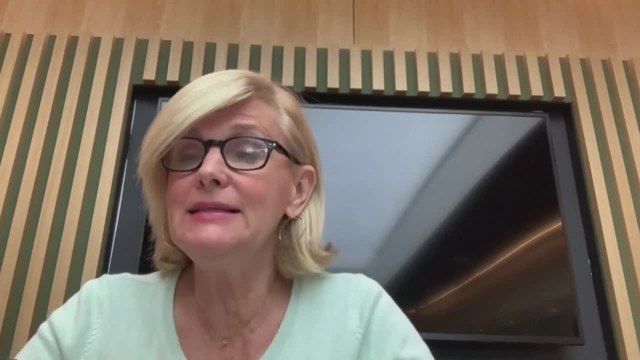 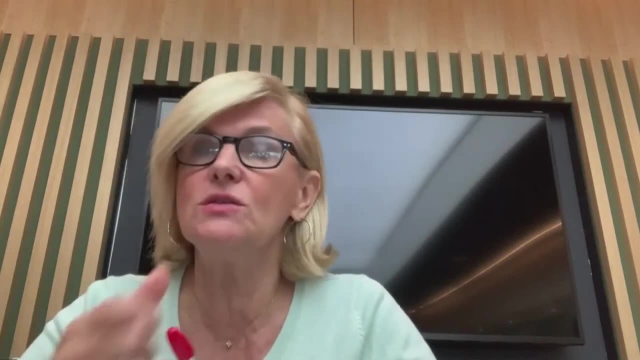 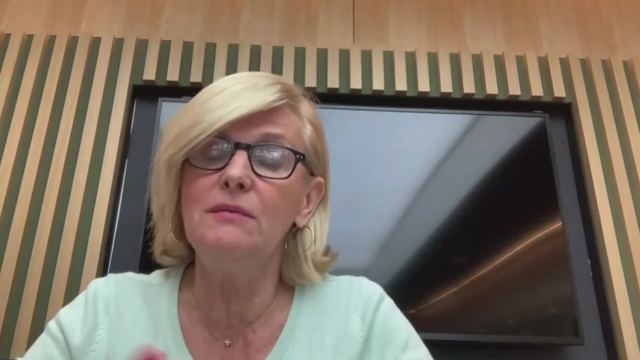 for the people. Gracias Gabriella. Yes, this is an issue that we are looking at under the occupational health standards. As you know, there are some recommendations now for outdoor workers and that will include these type of guards, or even, very recently, in Madrid as well. 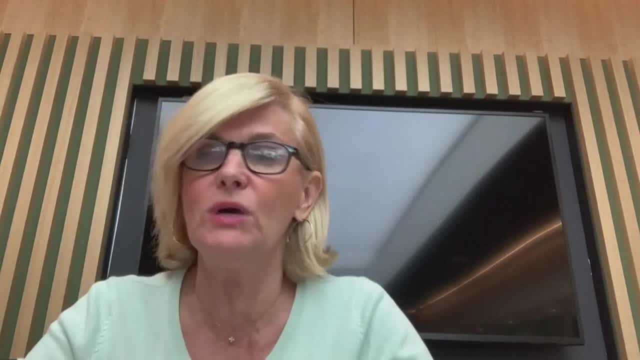 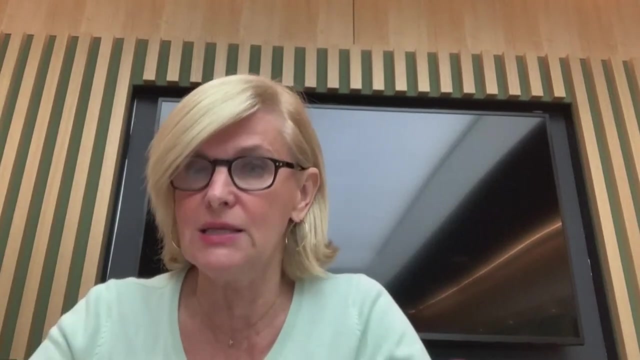 One of the cleaning outdoor workers. they were wearing a type of clothes that definitely will even increase the body temperature. So we are issuing recommendations about occupational health standards for outdoor workers And that's very important. How much the guards and the very heavy traditions. 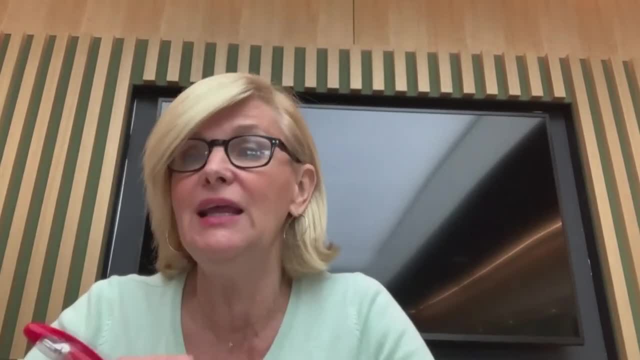 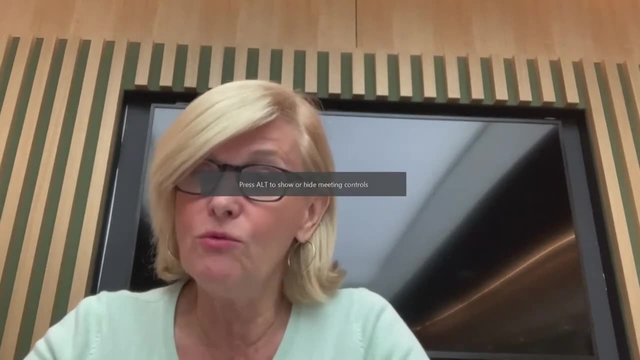 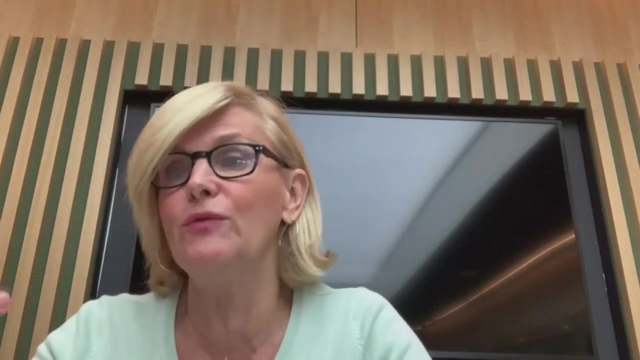 will be receptive to change in that, But definitely, if we are seeing this trend in terms of increase on the hip weights, our dress code needs to be adapted to that And we need to review the quality or the type of clothes we are using and making sure that it will be more adapted. 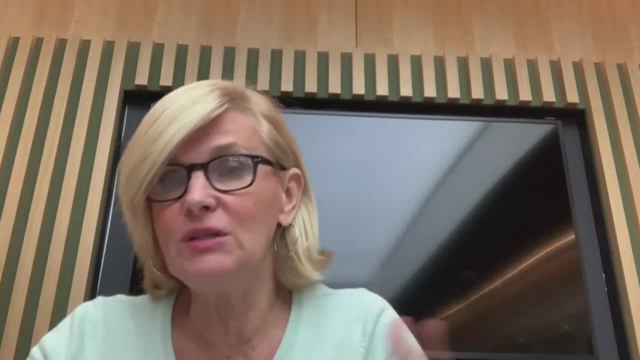 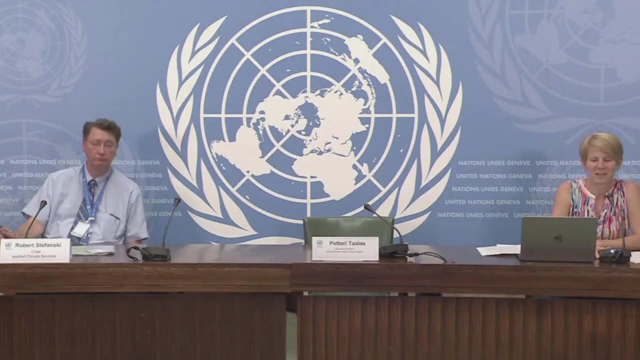 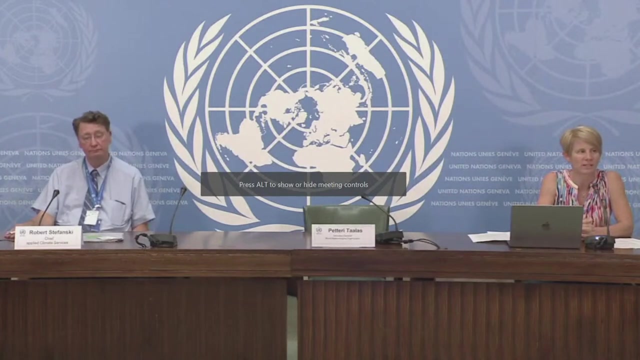 to the situation we are facing: The traditions. we hope that can be changed as well. Thank you very much. I think there are no more questions, So we will wrap up. Thank you very much for attending this press briefing. We will keep you updated. 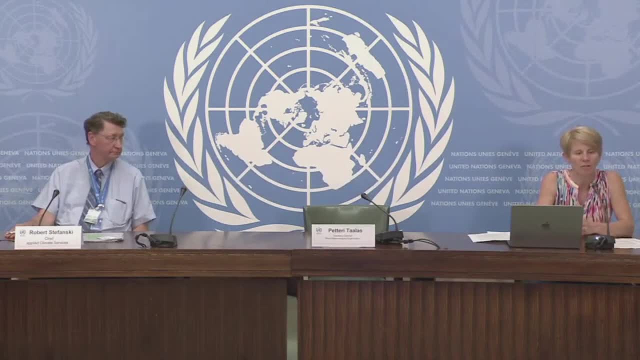 If you're interested in the naming of heat waves, we have published this morning an article on our website So you can get some additional information there, And the channel is open also with me. Don't hesitate if you want to get in touch.